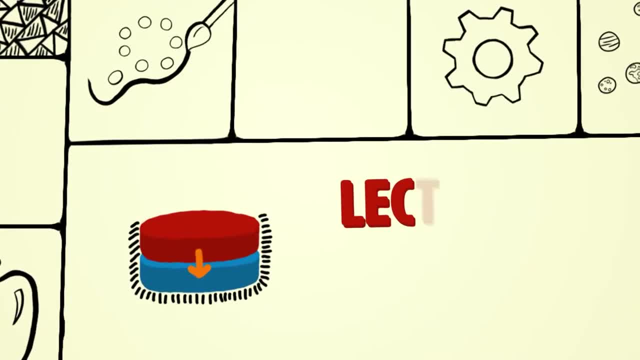 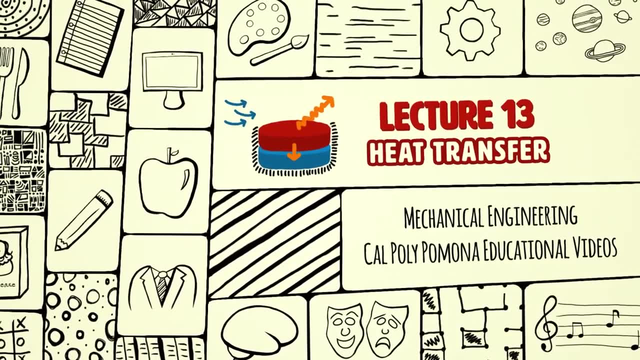 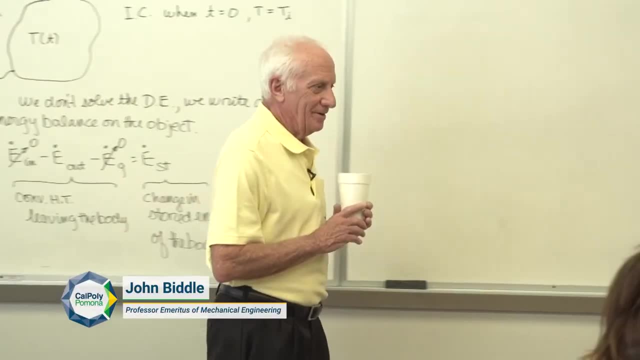 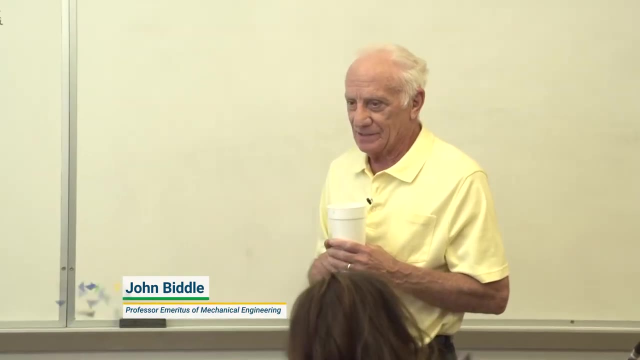 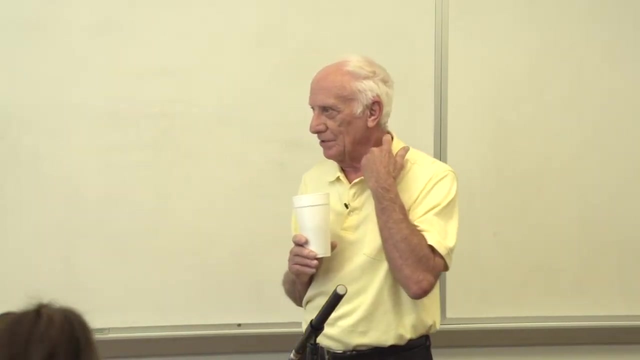 Heads up of where we are. We're starting a new chapter this morning, Chapter 5, which is the last of the four chapters on heat conduction. We're going to finish about half of that this morning and the rest of it on Monday after our first midterm. 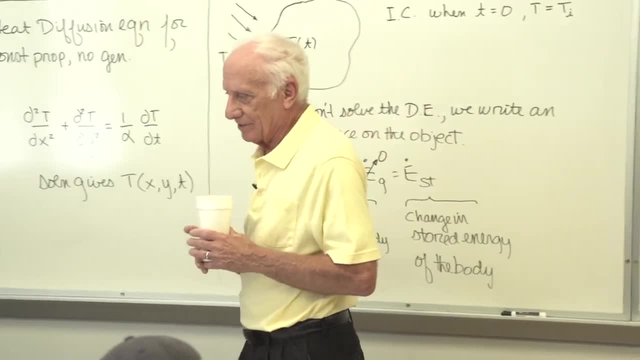 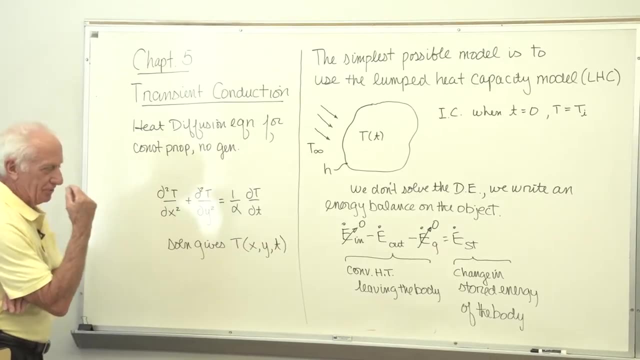 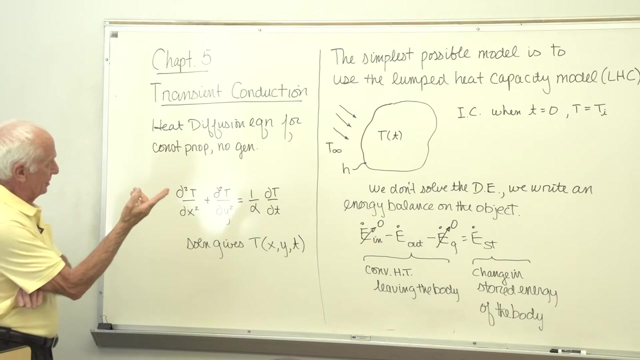 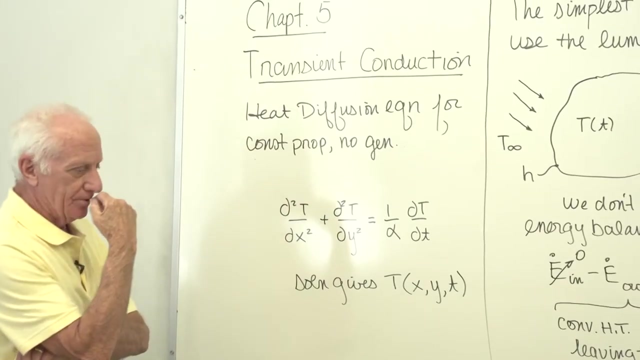 This chapter is titled Transient Conductions, So now time becomes one of the variables in our solution. We go back to Chapter 2 in general to get the heat diffusion equation in two dimensions. We write it here for constant properties with no generation. 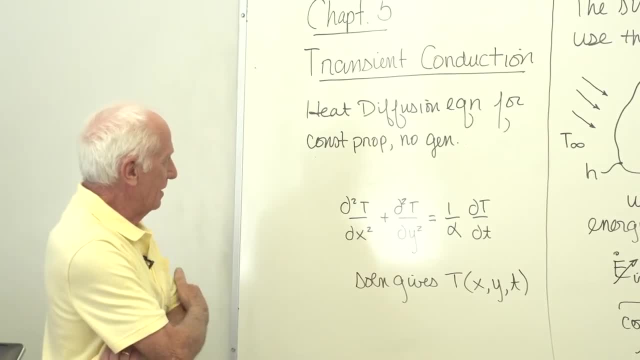 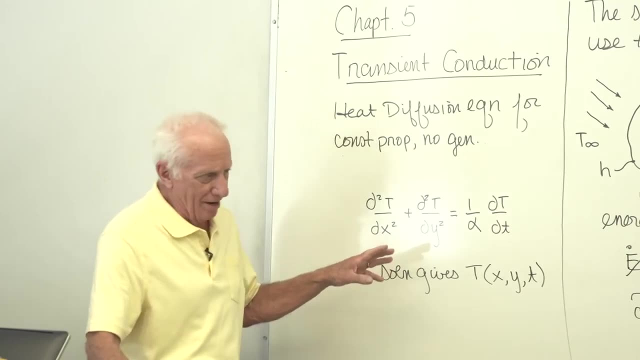 So this is the heat diffusion equation from Chapter 2, with constant properties, no generation. If we could solve this with correct initial and boundary conditions, we would get the temperature as a function of x, y and time. Now it can be rather difficult. 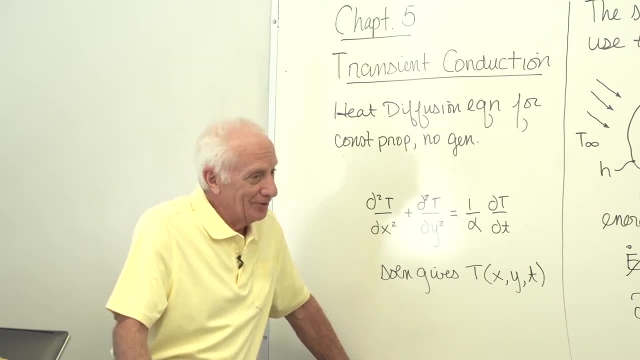 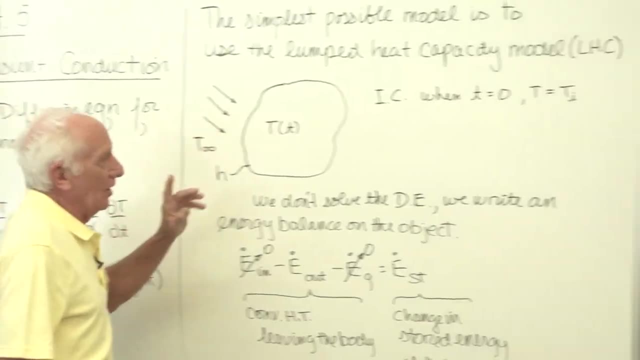 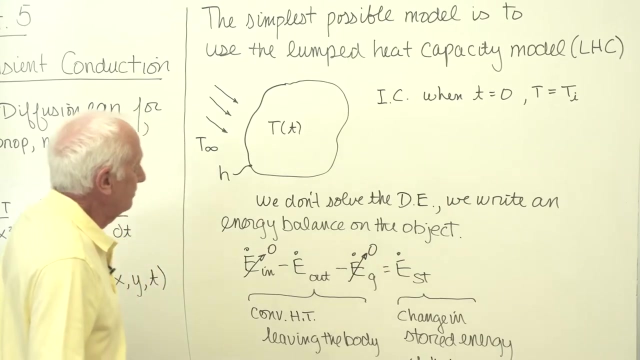 But luckily there is a possibility. we can use a simpler model to get results. This model is called the lumped heat capacity model, abbreviated LHC, lumped heat capacity. Here's what the model says: Take a body initially at a temperature Ti. 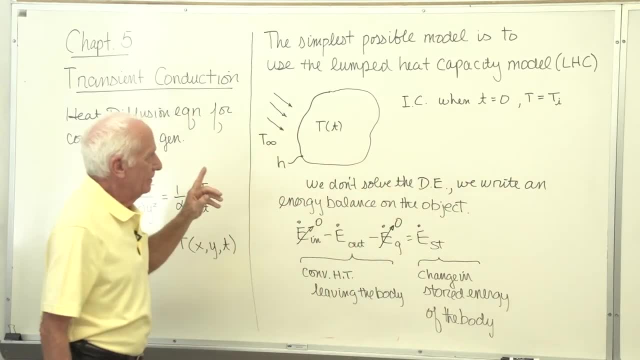 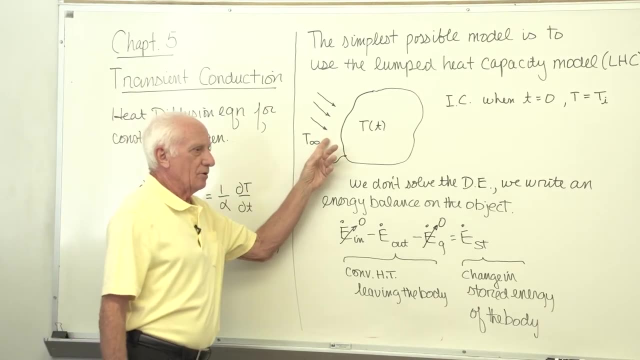 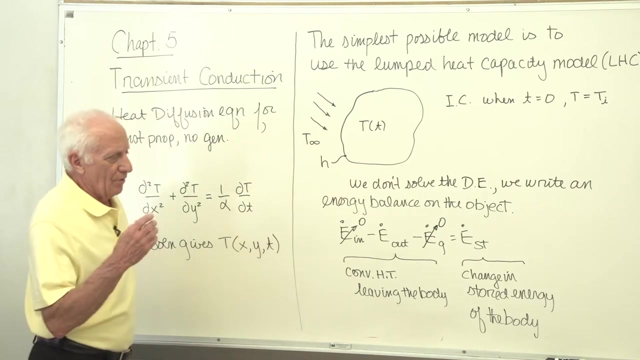 initial temperature at time zero Ti. Let's say it starts out hot. just to talk about something, It starts out hot. We blow a cool fluid over it at T, infinity with a convection coefficient on the surface of H. With time the body starts to cool, starts out hot. 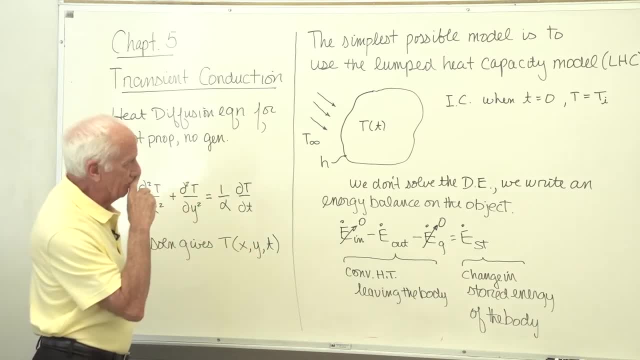 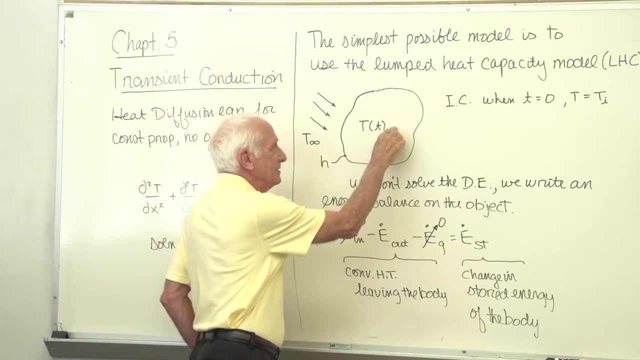 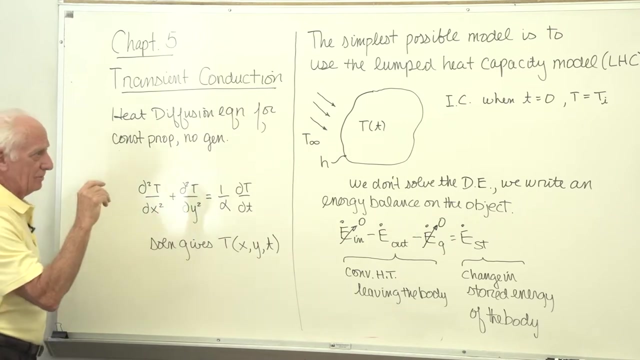 Blow cool fluid over it, temperature of the body starts to decline. We're going to assume with this simple model that the temperature does not vary inside the body with x and y, but it only varies with time. So now time is not a function or temperature is. 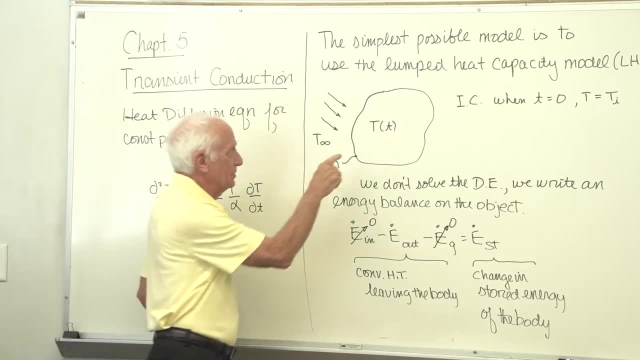 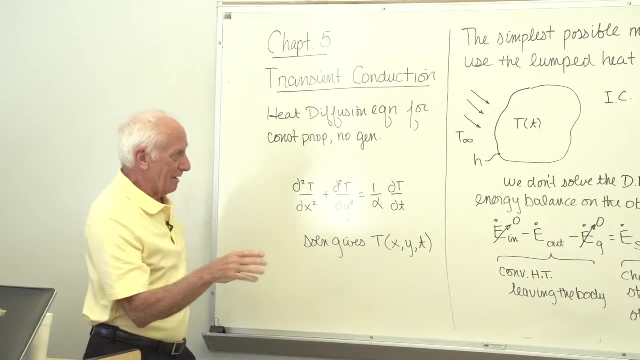 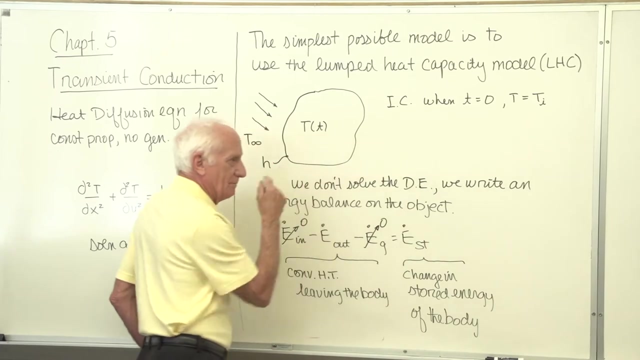 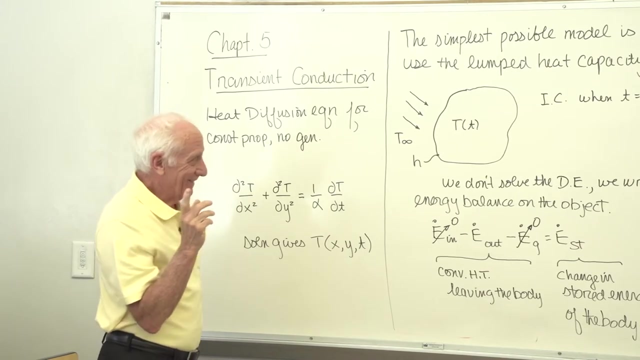 not a function of x, y and time. Now, temperature is only a function of time. We're not going to solve the differential equation now. Instead, we're going to write an energy balance on this object. So go back to chapter 1,. 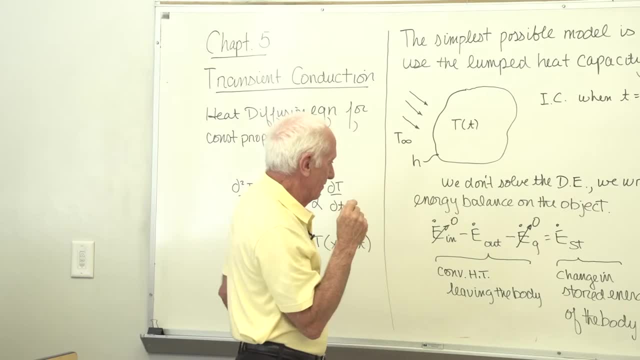 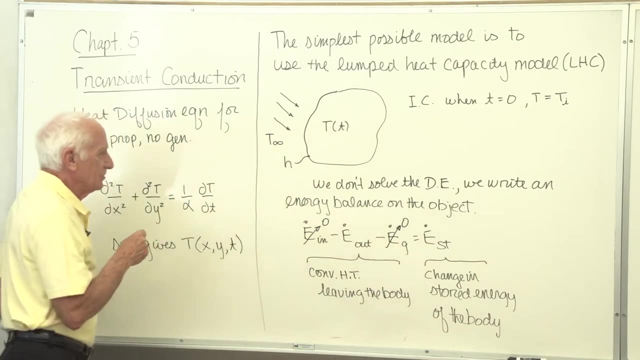 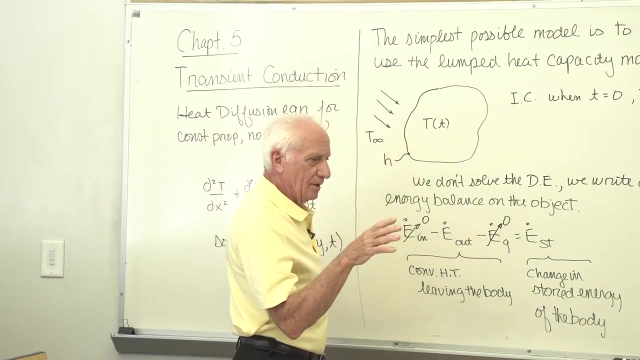 the end of chapter 1, energy balance on a control volume: E dot in minus E dot out minus E dot g equal E dot storage Problem said no generation E dot g zero. I'm looking at the model where the object starts out hot. 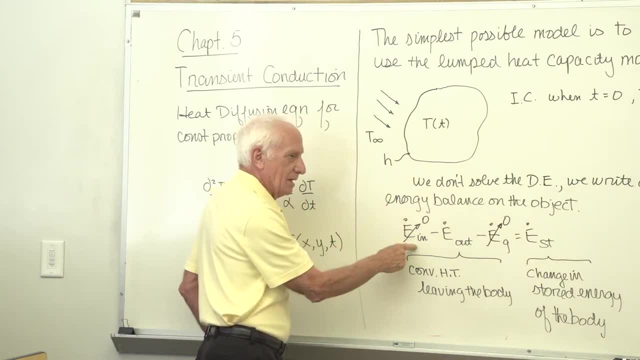 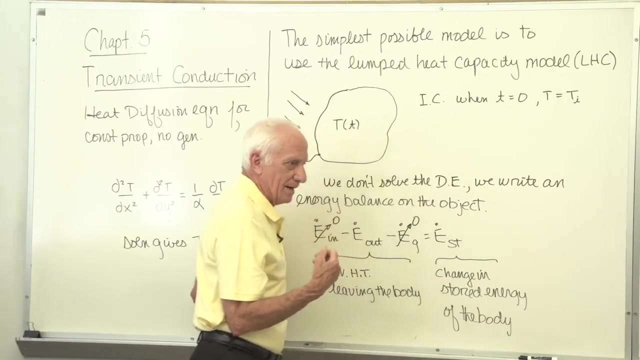 is going to be cooled by a colder fluid, So nothing comes in, But energy does go out by convection. There's a convection leaving. What happens then? The body has a change in stored energy. We're taking energy out of the body by the cool fluid blowing over it. 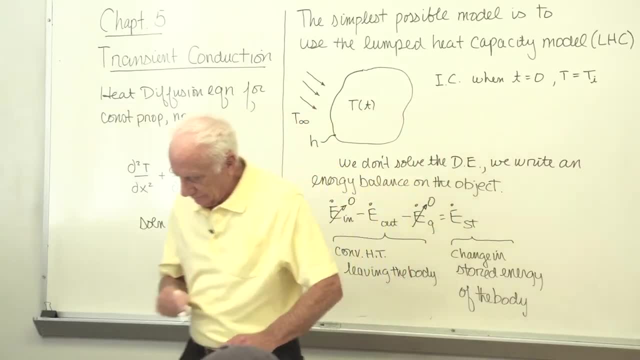 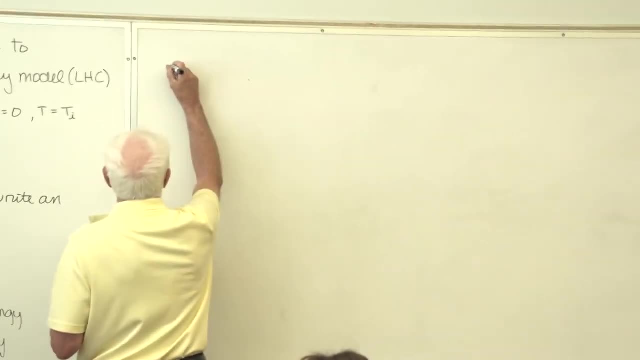 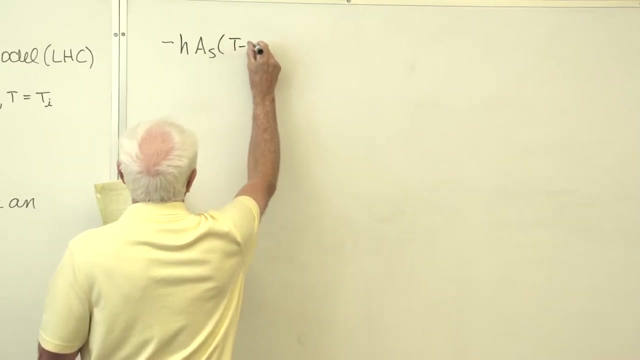 So we can then write down what the convection is and the change in stored energy. So we have convection minus h A, S and T minus T- infinity. Just to review chapter 1, convection, heat transfer, Newton's law of cooling. 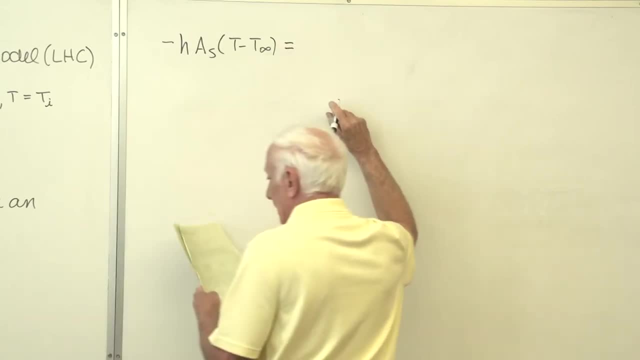 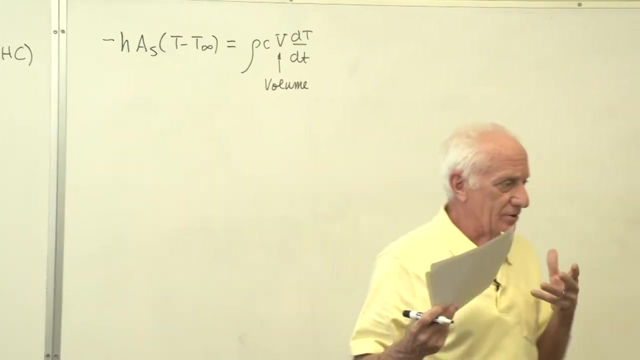 equal the time rate of change of stored energy. Rho C, V, dT, d time Capital. V is the volume Rho times the volume is the mass. The mass times C gives me a measure of how much energy the object can store. 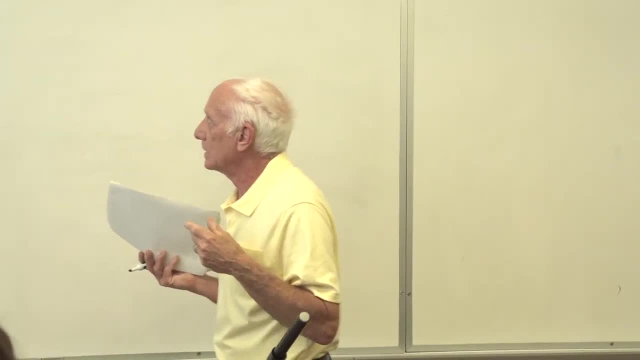 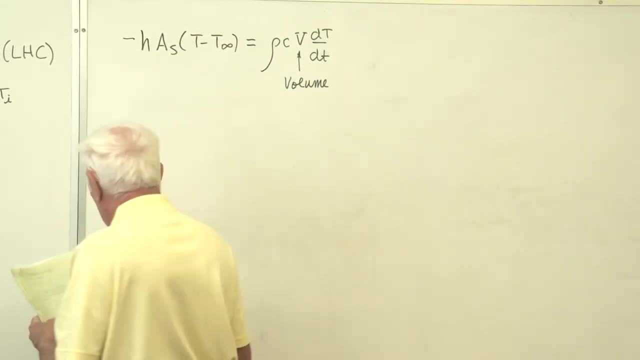 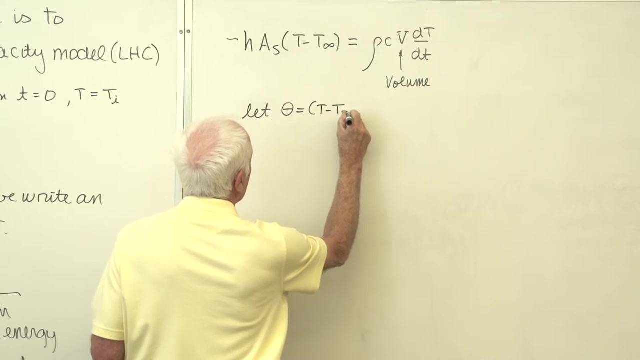 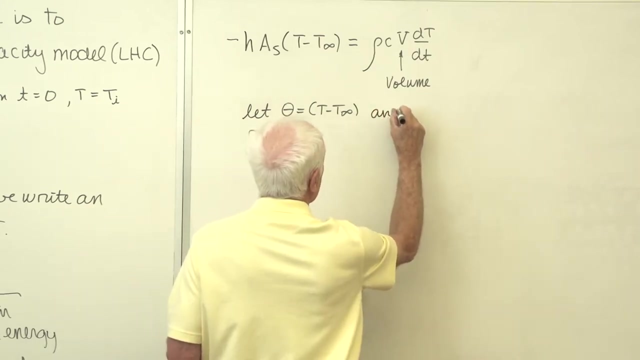 Mass times. C, specific heat. Units of the equation. there are in watts both sides of watts. To simplify matters, we let Theta equal T minus T, infinity. Put that in the above equation, then well, what happens, of course, is d theta. 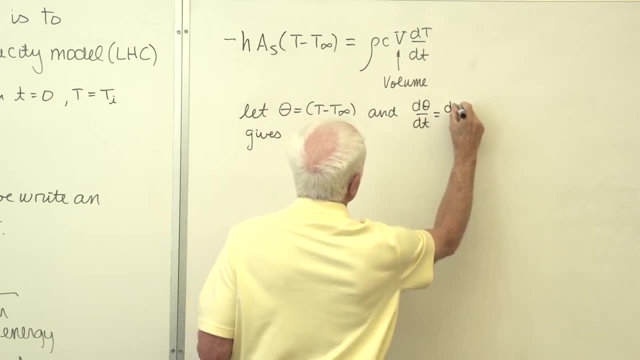 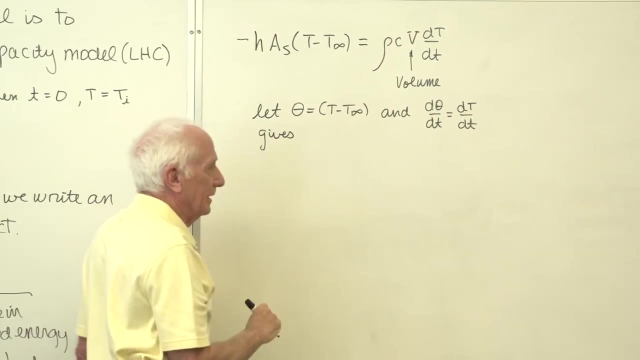 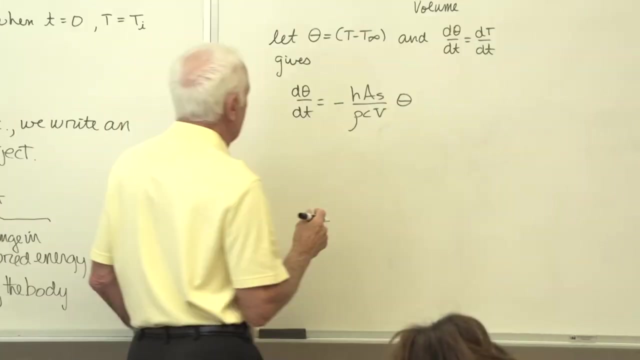 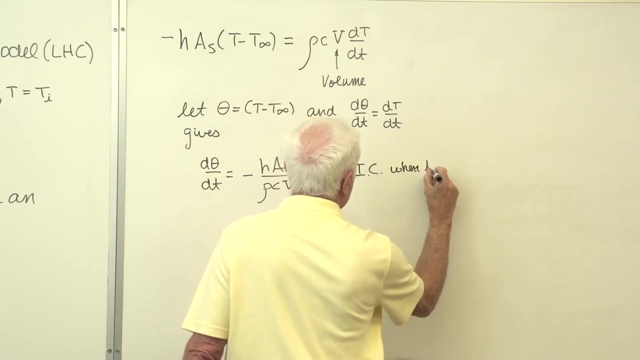 d theta. dt is equal to dt, dt, Because a differential of a constant t- infinity- is zero. Put that up there, So we'll write it down: d theta over t. There's our little differential equation. The initial condition is when t equals zero. 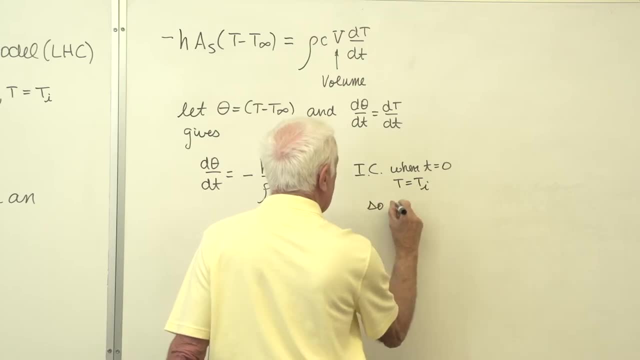 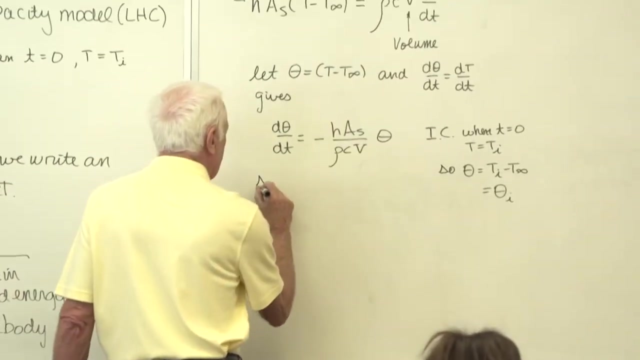 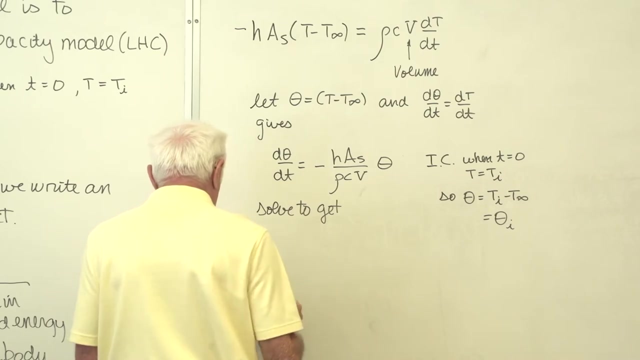 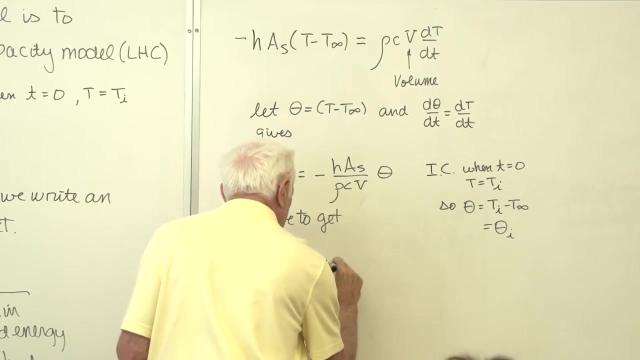 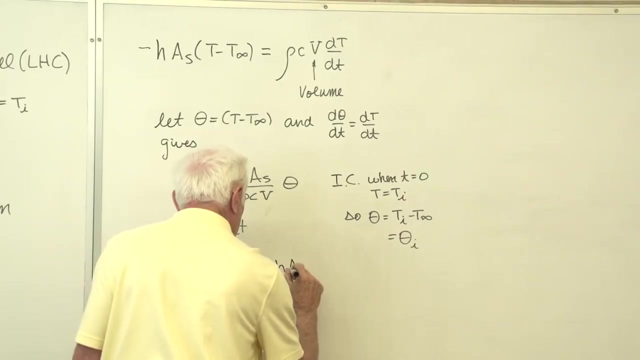 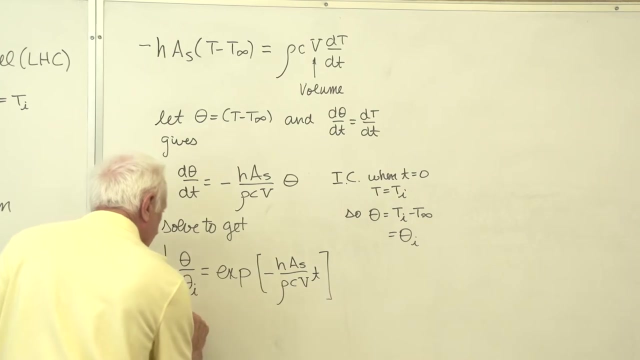 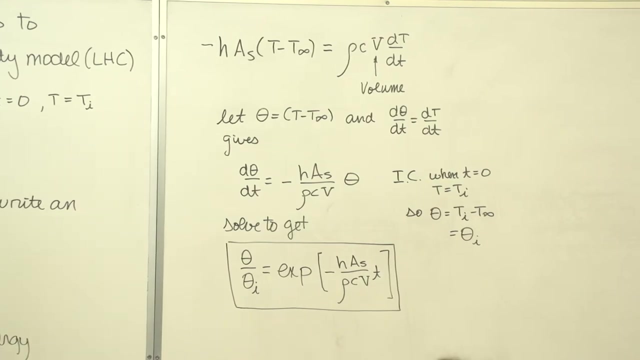 t equal ti, So theta is equal to ti minus t, infinity and we call that theta i. So when time equals zero, theta equal theta i, a constant, Solve then theta over theta i. We get that solution for temperature of the object as a function of time. 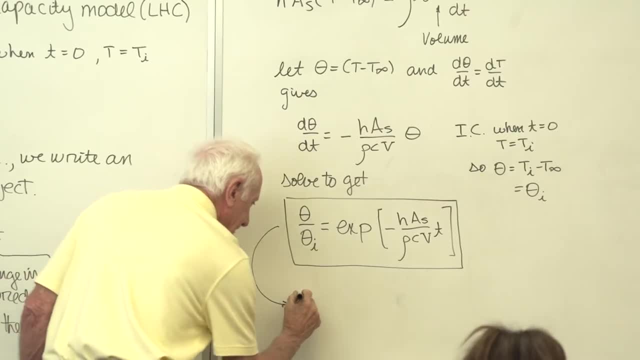 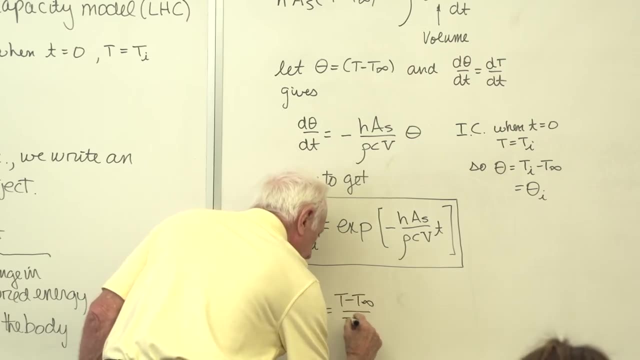 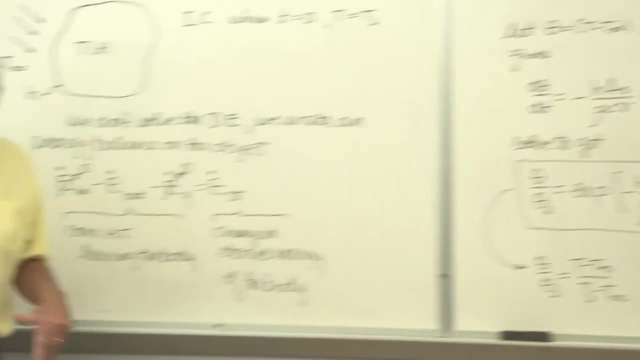 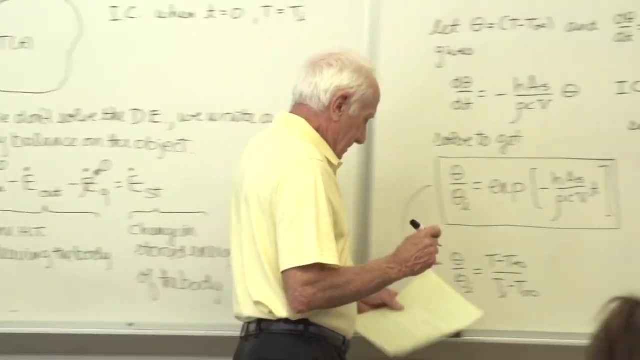 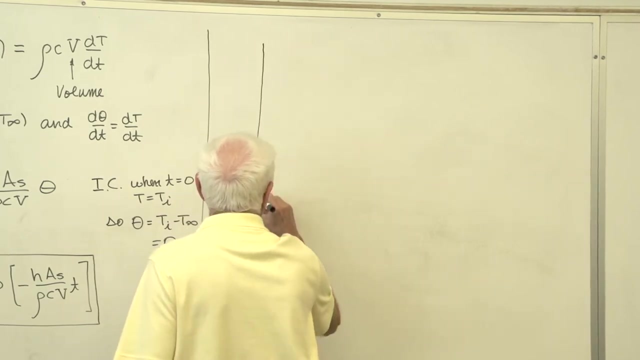 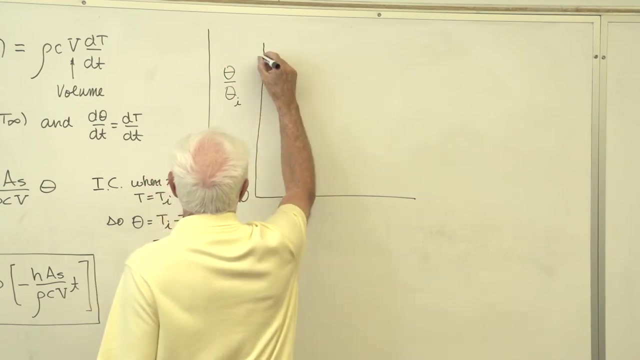 Now just to remind you what theta over theta i is. So theta over theta i is a measure of the temperature, And if we want, then we could plot a curve of theta over theta i from zero to one. And this is time. Start at one. 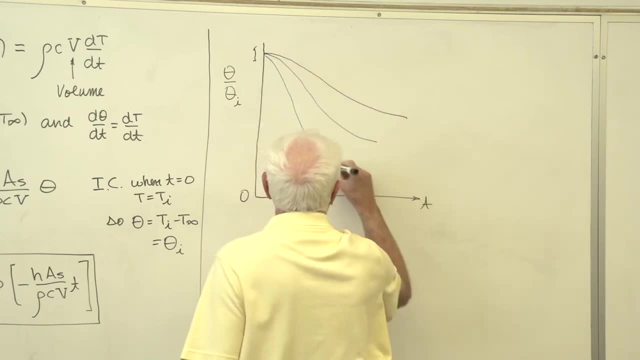 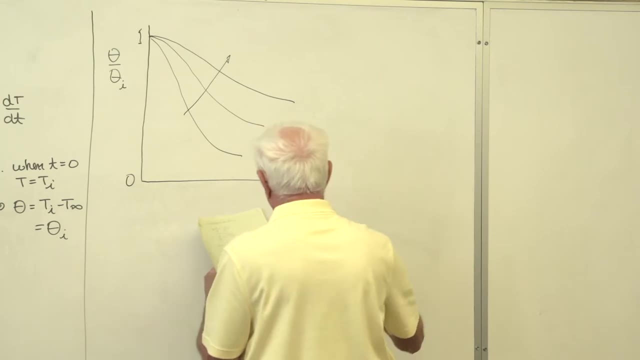 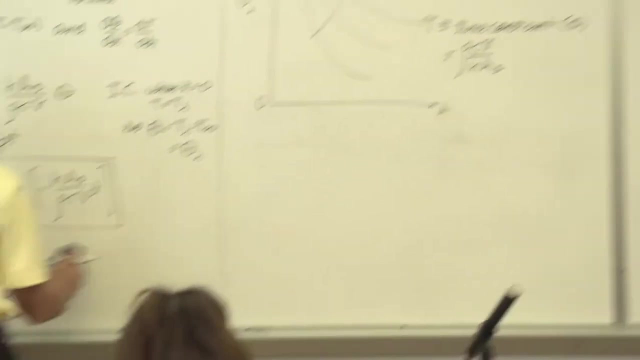 And there's different curves, Parametric values. Each particular curve is a different value of the time constant called tau. It's in seconds, It's rho, cv over h as, So if you want, I'll just add this to it. You might want to express this as exp. 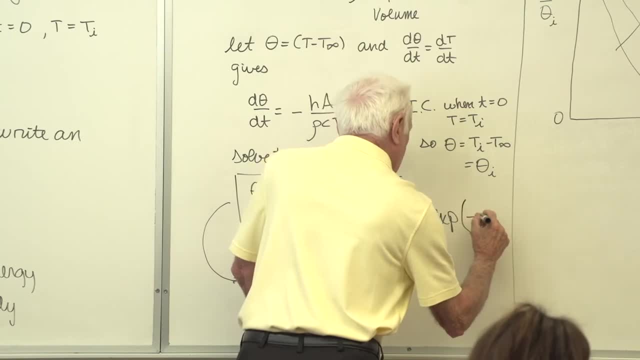 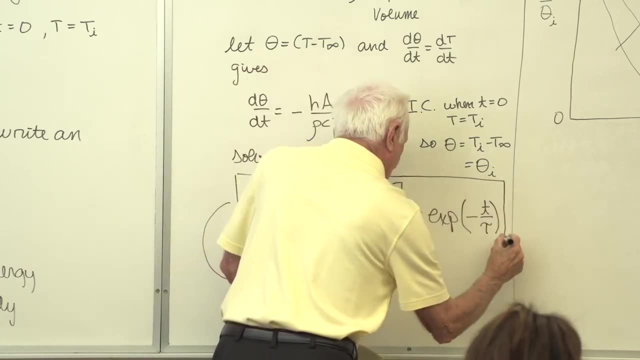 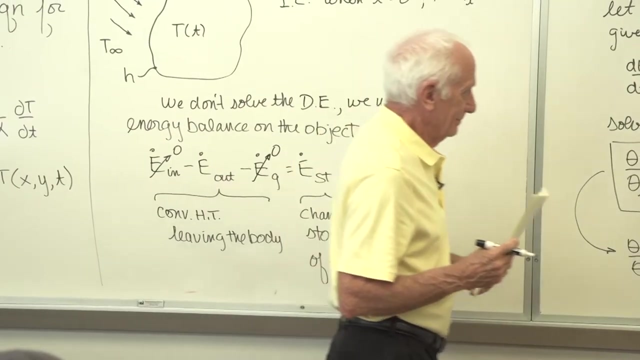 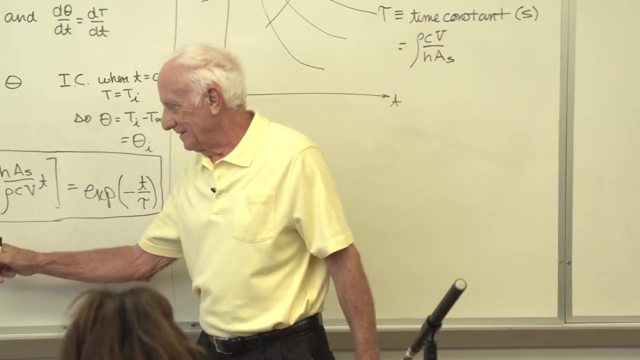 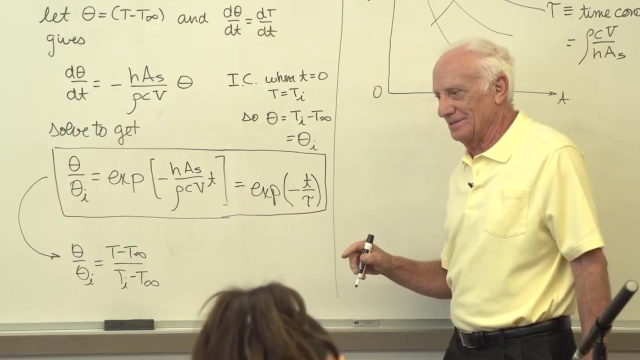 It's a simplified form of this. then, minus t over tau. We engineers love the dimensionless stuff. This is a dimensionless temperature difference ratio. This is dimensionless. T over tau is dimensionless. T is in seconds. Tau is in seconds Dimensionless. 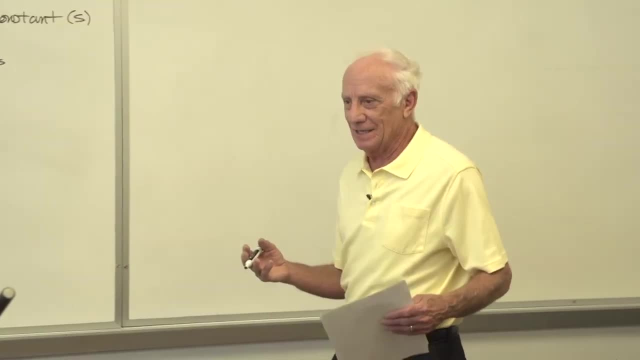 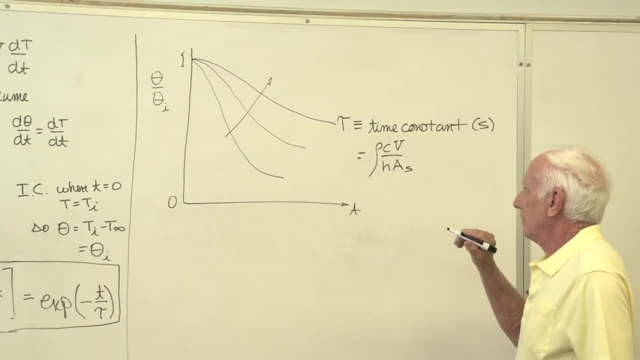 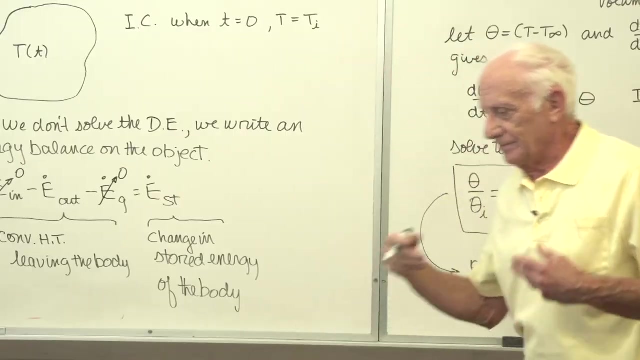 So we like to express things very simply, and a lot of times that's in dimensionless form. But this is called the time constant tau. Now let's just for sake of talking about something. let's just take a copper sphere six centimeters in diameter. 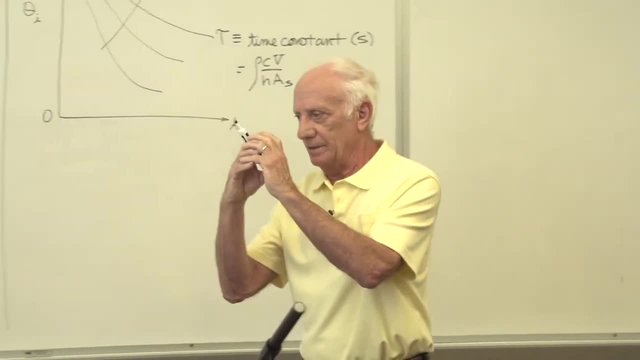 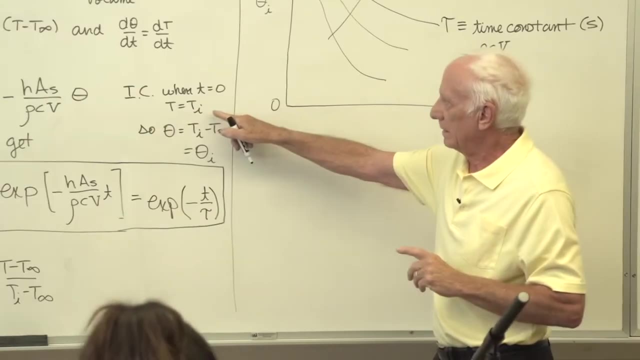 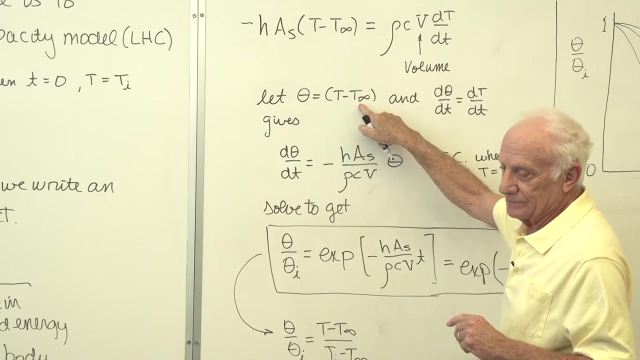 I don't know that size of baseball size, Six centimeters in diameter, Initially, at 300 degrees Fahrenheit, That's Ti 300. I'm going to blow air over it at 30 degrees Celsius, Not Fahrenheit, Let's say 70 degrees Fahrenheit. 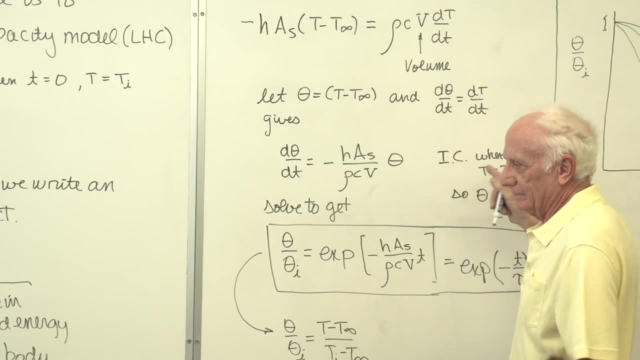 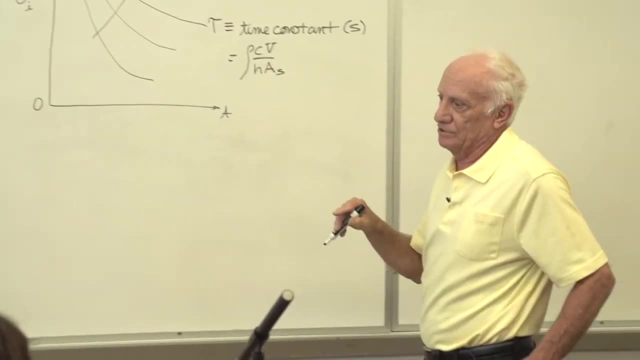 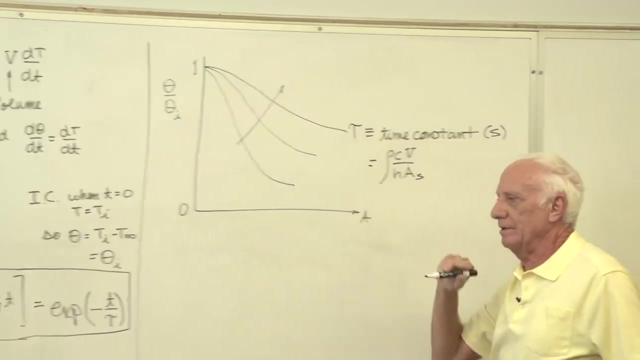 make it English units, So 300 degrees Fahrenheit initial, and now T infinity, 30 degrees Fahrenheit. I blow air over it. Of course the temperature is going to drop with time. How Exponentially Drops with time, exponentially. But these three curves, 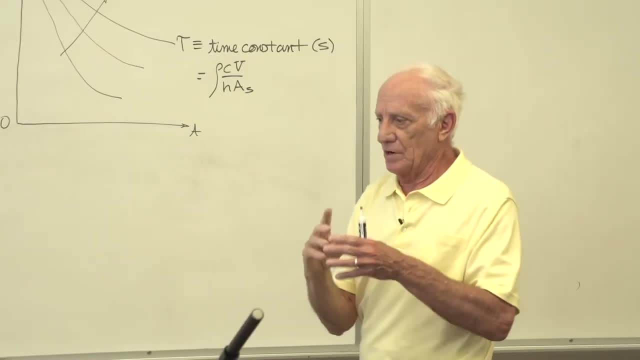 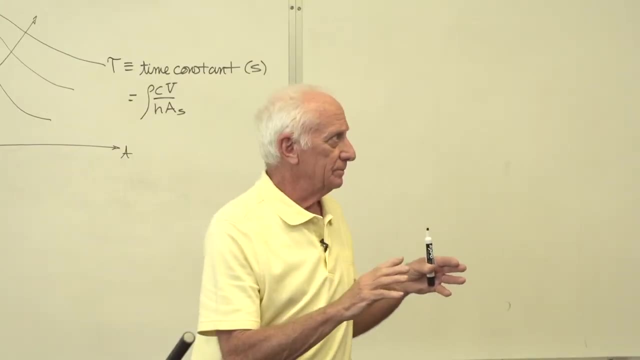 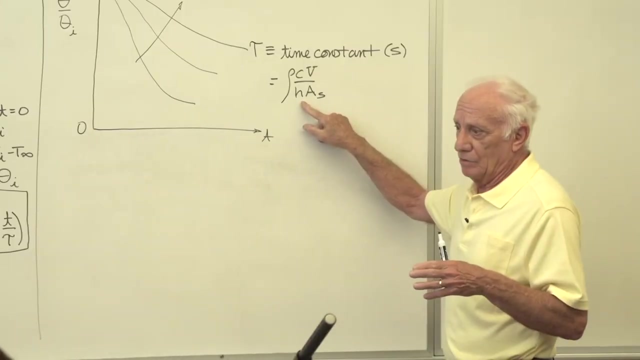 let's say, you take that copper sphere and put it in this room on a stand at 300 Fahrenheit. The air in this room is really still. Nobody's hair is blowing. The air in the room is really still. H is going to be really low. 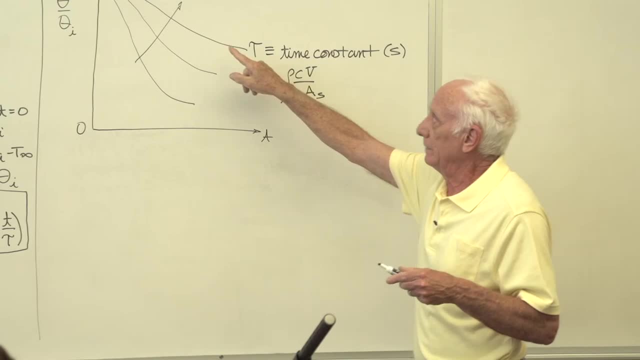 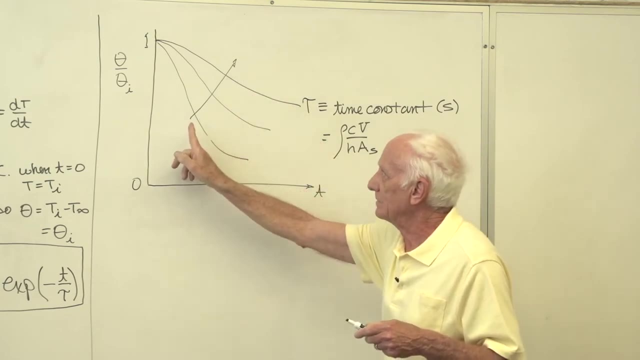 Time constant is going to be really high. This arrow means high time constants, low time constants. The direction of the arrow tells me Increasing time constant curves this way. So copper sphere in this room. it cools real slow. Now I put a floor fan in front of it. 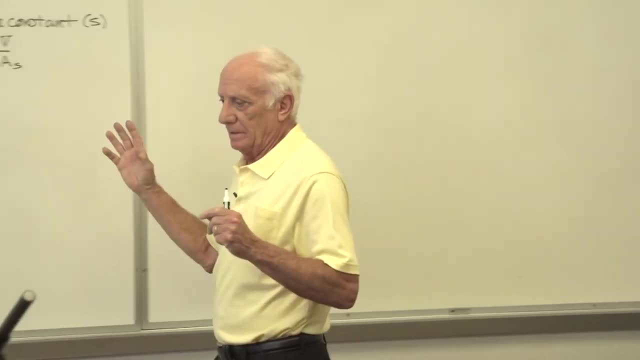 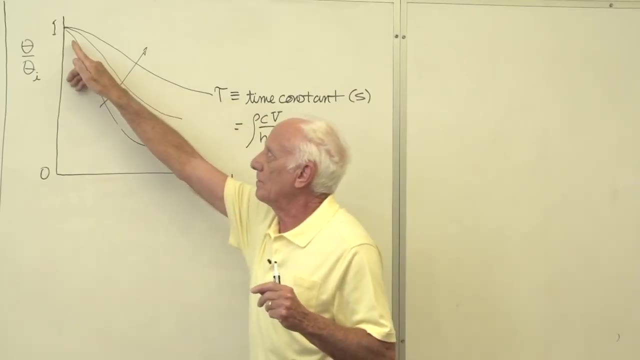 Turn the floor, fan on. the air blows by really fast. H becomes really big. H really big Time. constant, really small. Oh boy, the temperature drops really fast in that copper sphere. So that's the story this graph is trying to tell you. 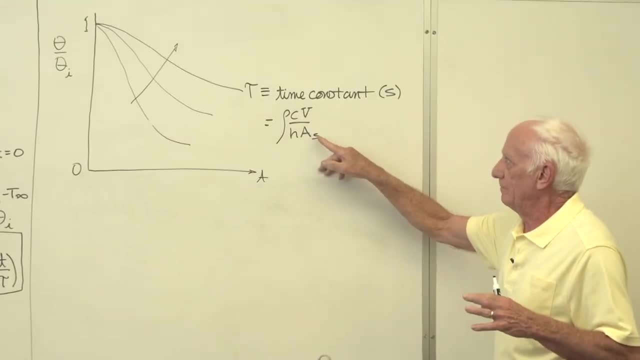 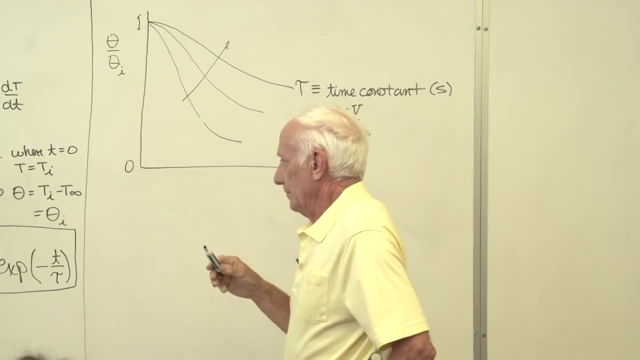 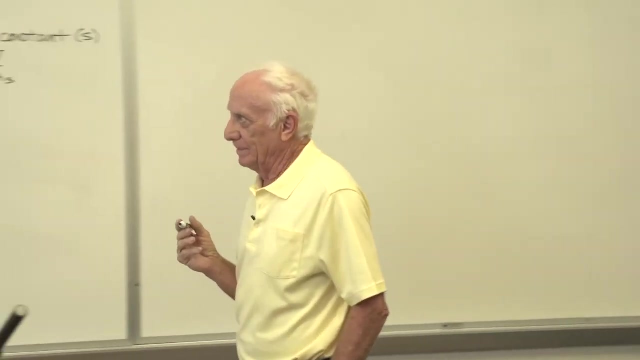 You can say: what if the density is bigger? What if the surface area is smaller? You can play the same game with all these variables. So there is the temperature variation with time. Very simple, Because it's the simplest possible model that we can use in transient studies. 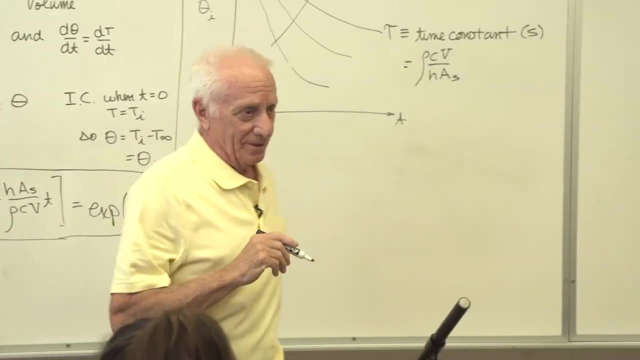 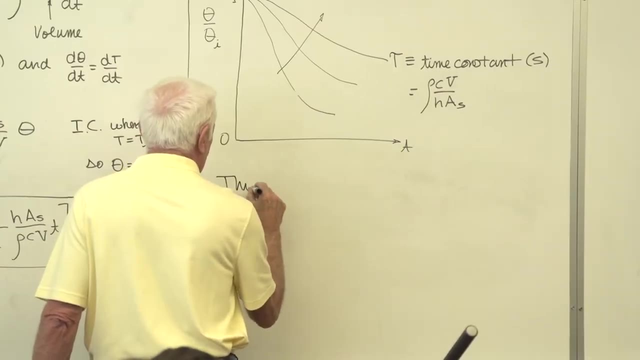 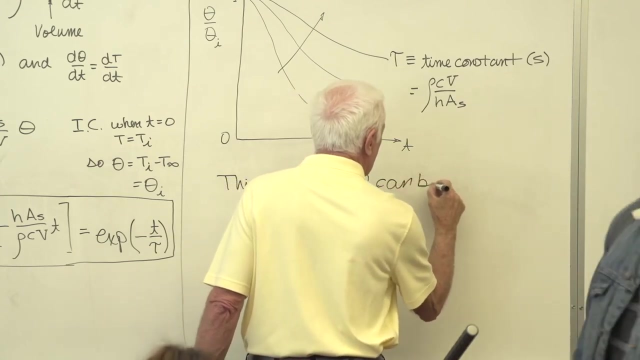 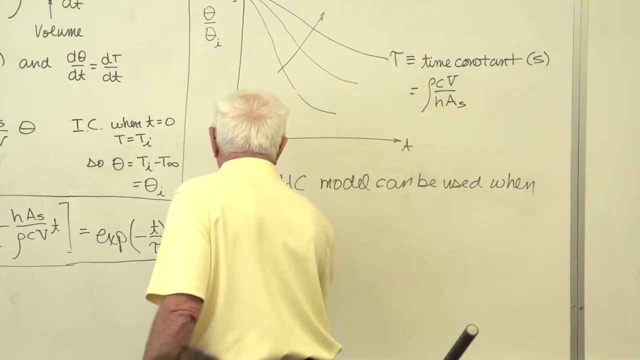 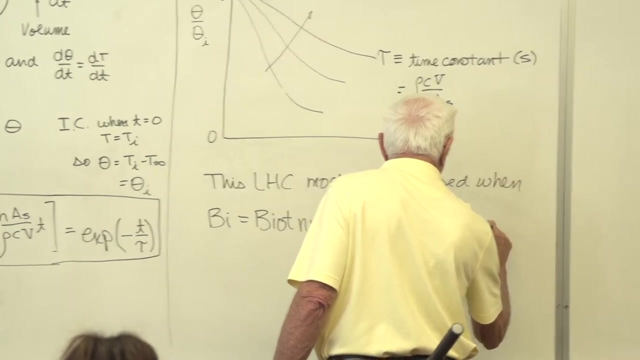 But now we say, yeah, but when can we use it? Okay, well, when we can use it is when something special happens. This lumped heat capacity model can be used when a dimensionless parameter called the Biot number, defined as HLC over K, is less than one-tenth. 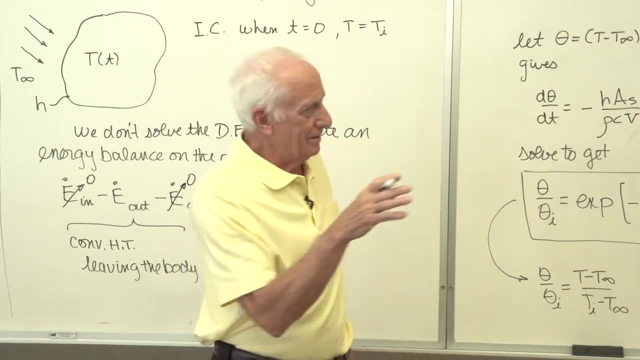 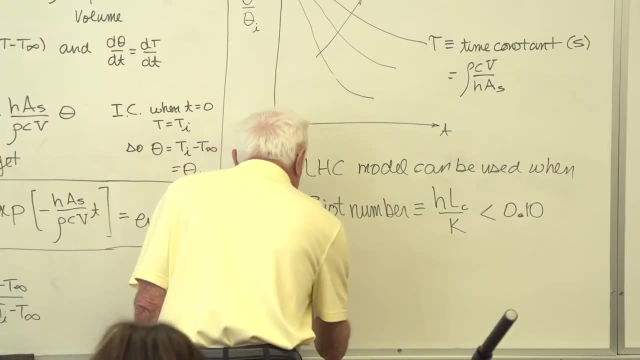 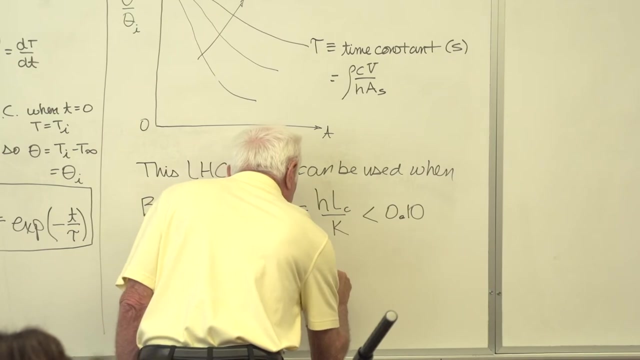 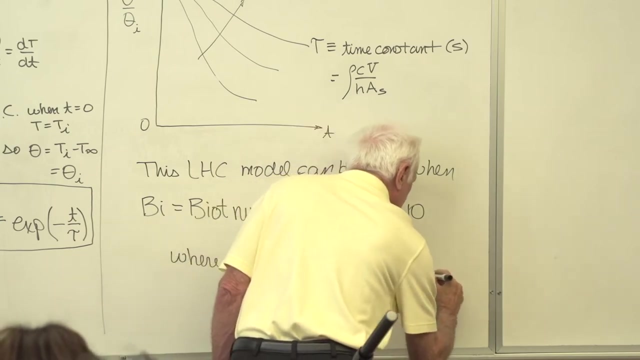 If that's satisfied, we can take the easy way out and model the problem as a lumped heat capacity model. What is L sub c? L sub c is called a characteristic length. It's the volume of the object divided by its surface area. 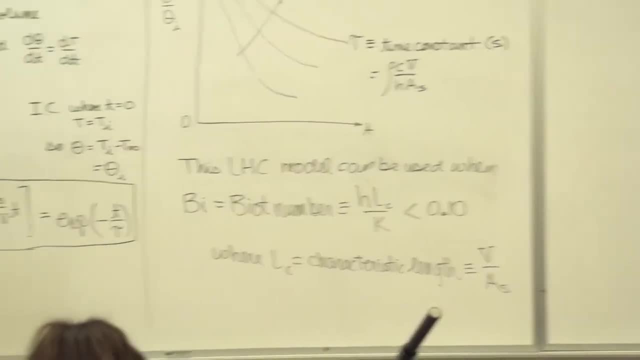 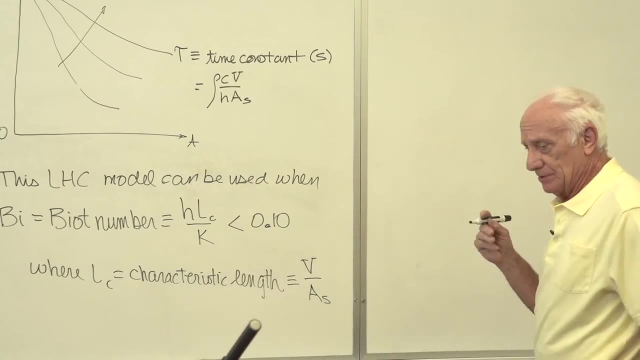 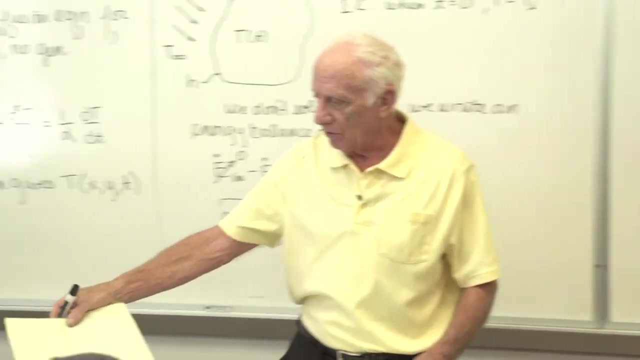 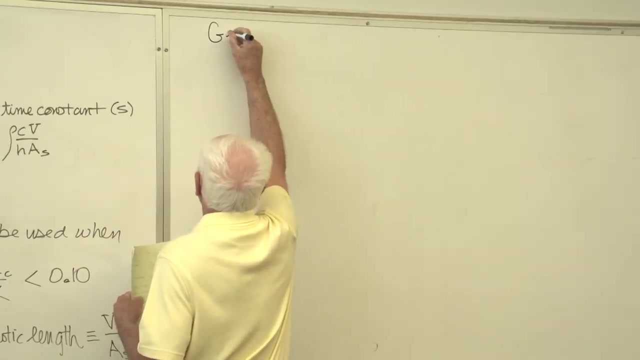 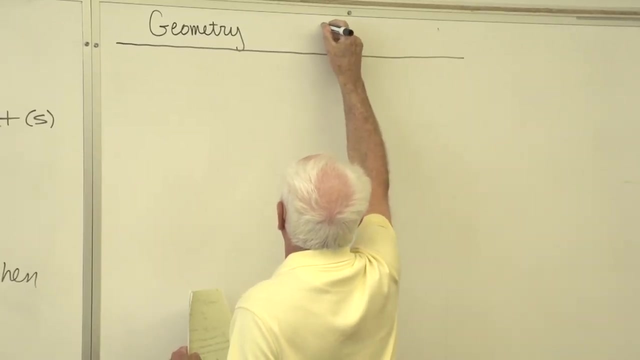 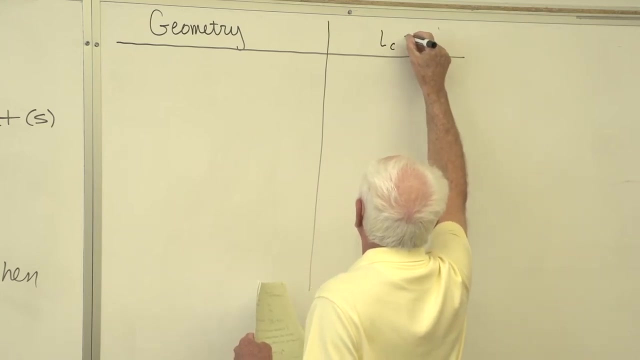 the area touching the fluid, cooling the object. So there's some simple geometries. We'll put those geometries up on the board here. The first one is a plane wall, Plane wall. This particular plane wall has convection on both sides. 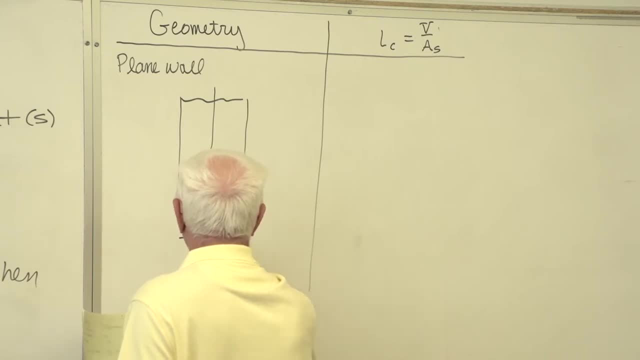 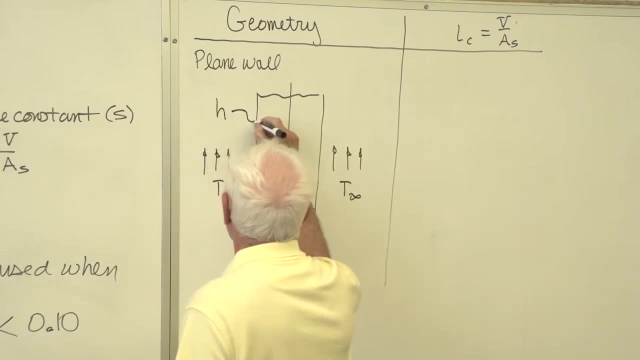 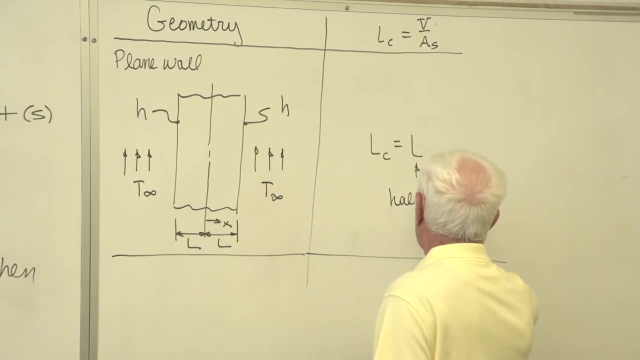 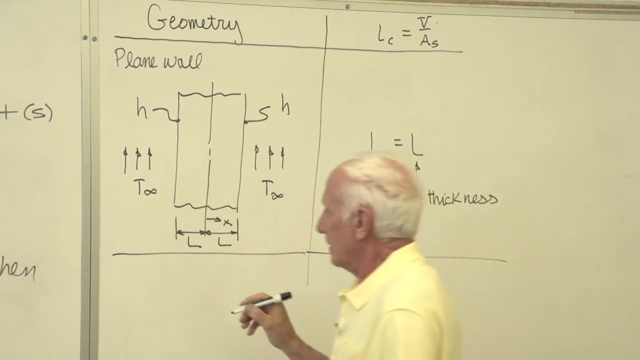 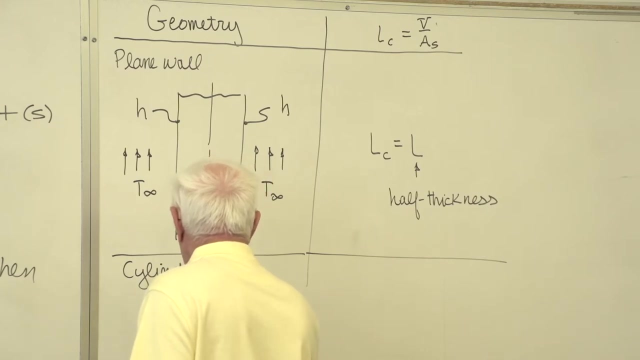 with a convection, coefficient of H, Lc is equal to L. It's called the half thickness. Another common geometry is a cylinder Whose radius is R. naught Again, it has a fluid blowing over it at T, infinity. with a convection. 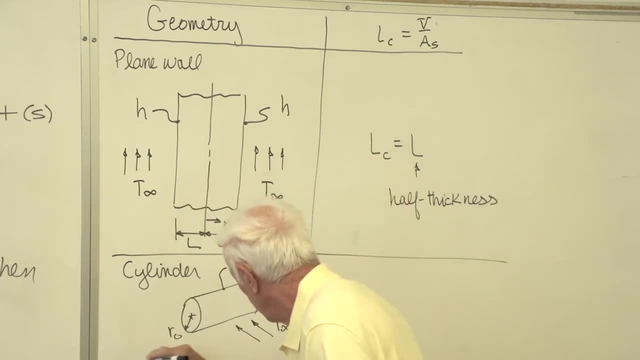 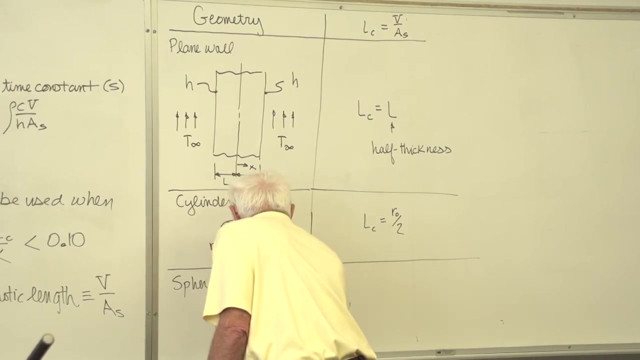 coefficient of H on the surface, For this case L sub C, equal the radius divided by two. Now we have a sphere Again. we have a fluid blowing over the sphere at temperature T infinity, with a convection coefficient H on the surface of the sphere. 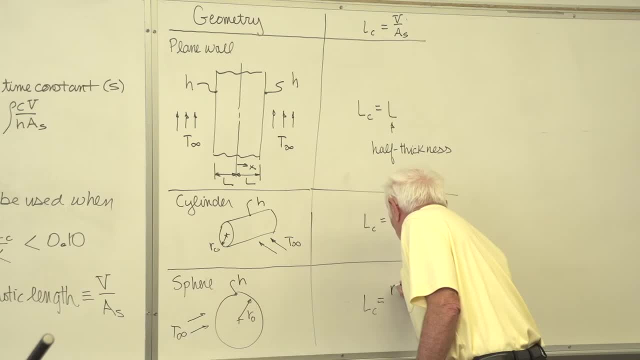 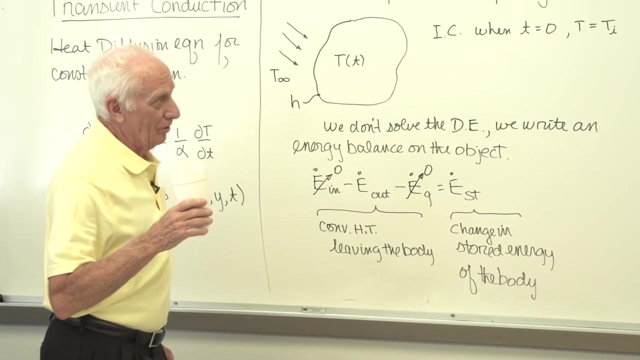 L sub C equal R naught over three. So those are three common common geometries that we engineers study. I'll tell you later on what give you some idea what they really could be, But for right now, plane wall, a cylinder and a sphere. 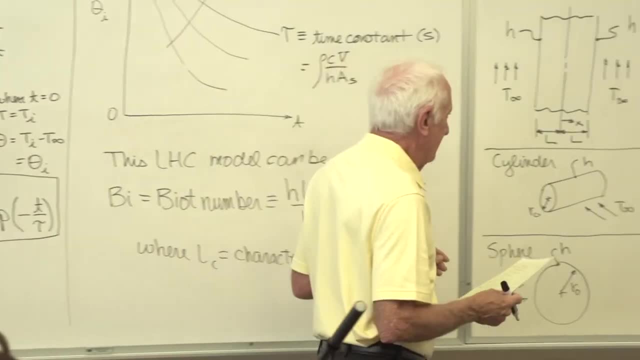 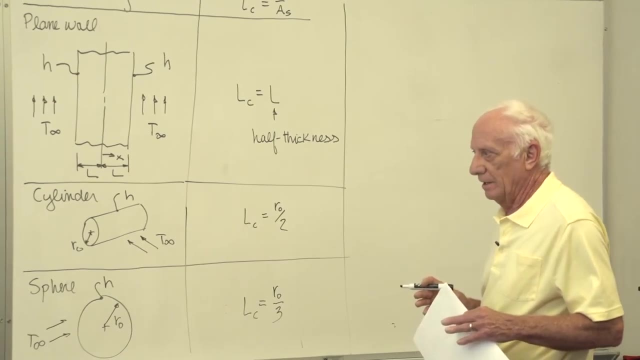 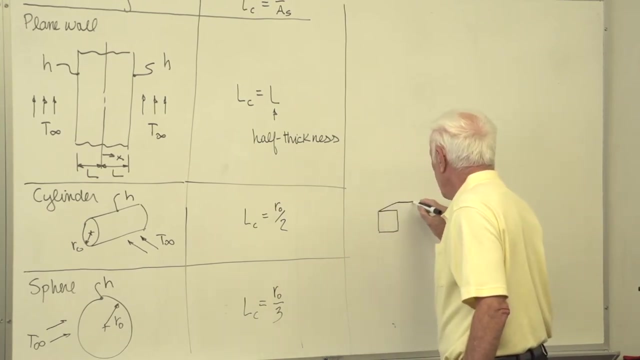 B, your number H. Lc over K. Here's Lc. I don't care what the object is, you can find Lc over K, Lc for it. For instance, what if I had a cube of aluminum? Cube of aluminum: each side A, L sub C. 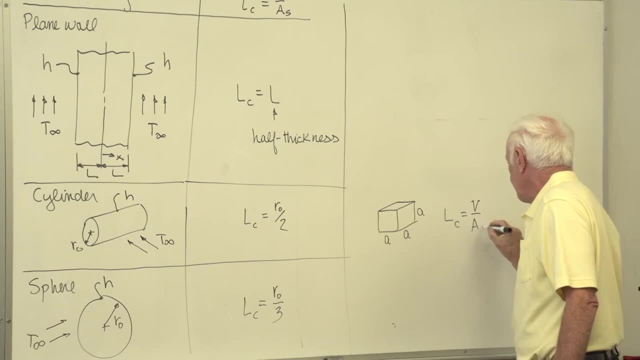 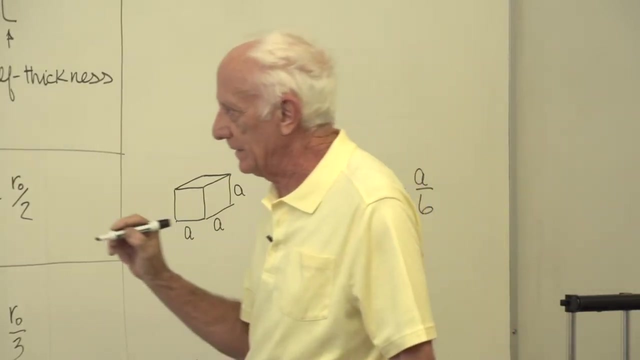 volume over surface area. volume A cubed. How many sides? Six? What's one side A squared L sub C length of one side divided by six? That's what goes in the B-O number. So for any object, 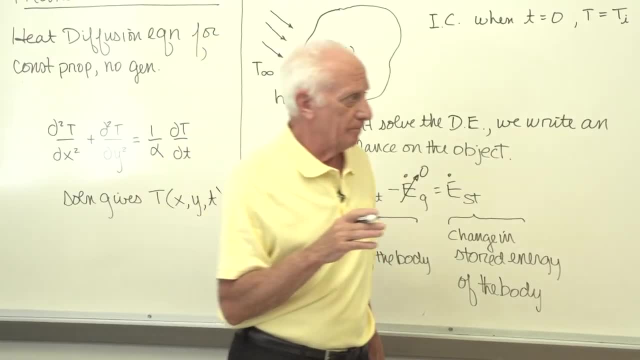 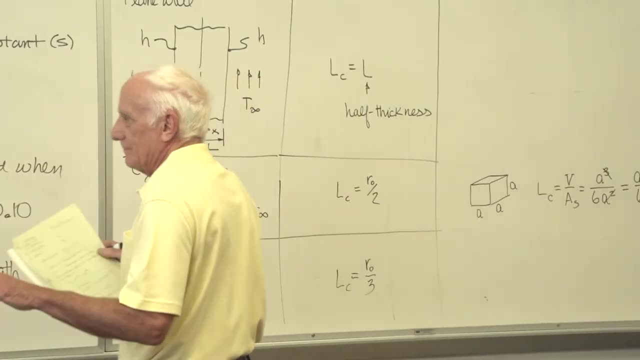 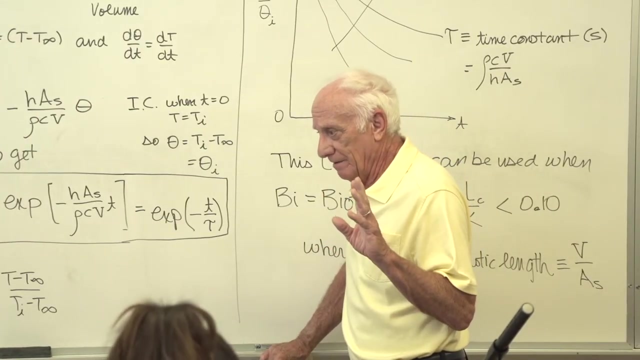 it's the volume divided by the surface area touching the fluid. All right, Well, that's half the story. We know the full story. The full story is once we get the temperature of an object, whether it's a temperature as a function of 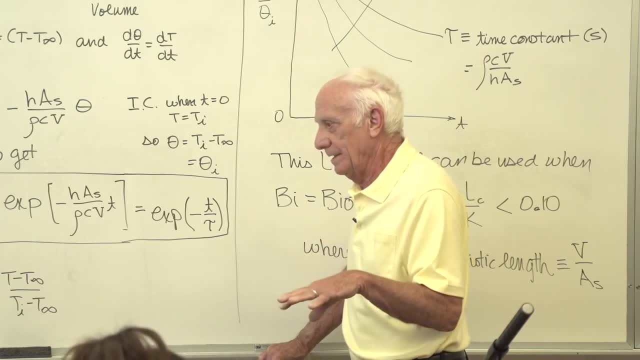 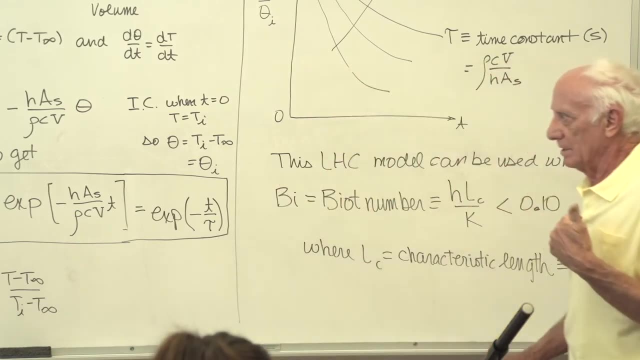 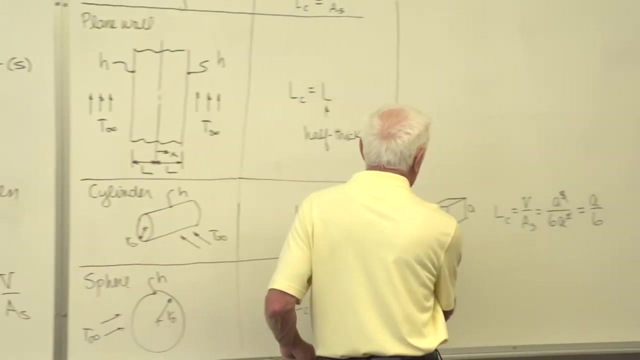 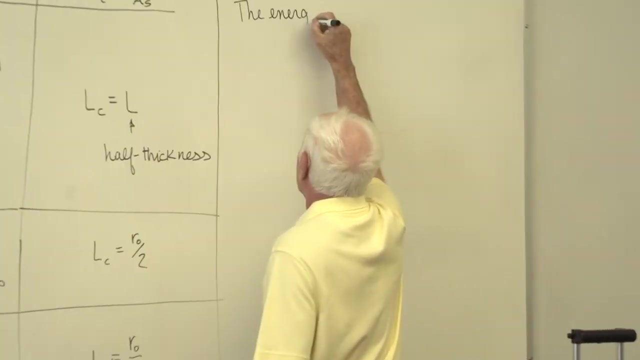 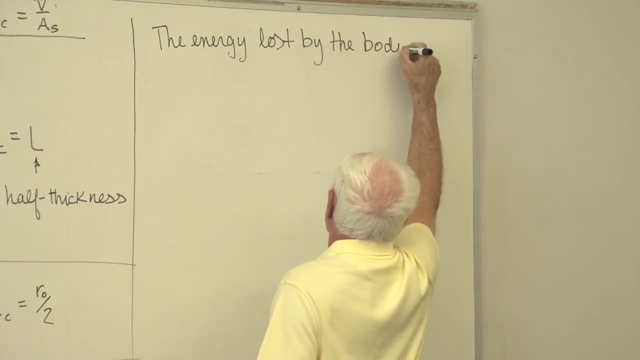 the geometry or of time. the second thing is find out something about how much heat transfer has occurred by convection or how much energy the body has lost by convection. So now we want to find the energy lost by the body. And how is that energy lost by the body? 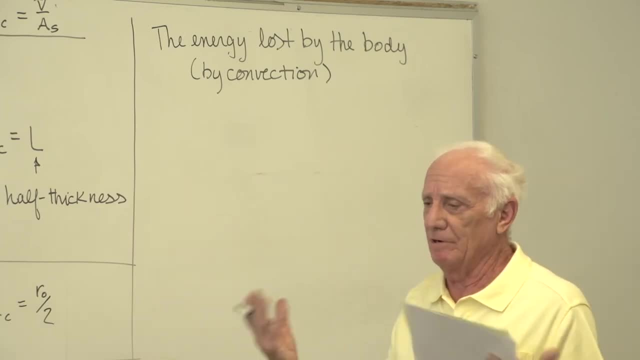 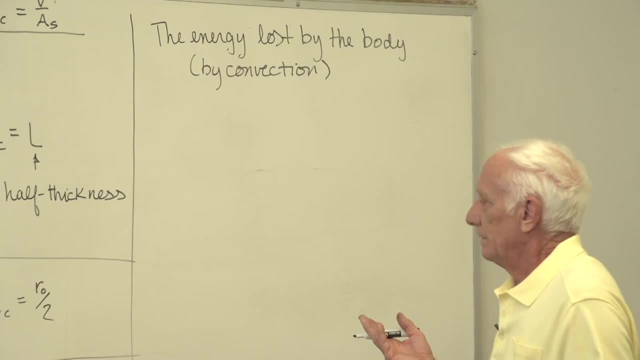 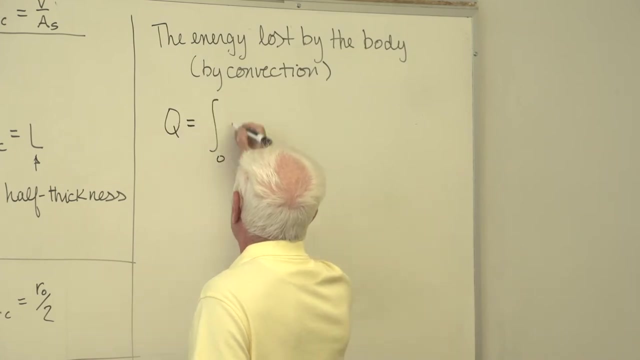 Well, convection to the fluid takes it out. Now it could be the reverse: Hot gas, initial temperature low, You heat the body. It doesn't matter either way, All right. So Q equal integral zero to time. T rho HAS. 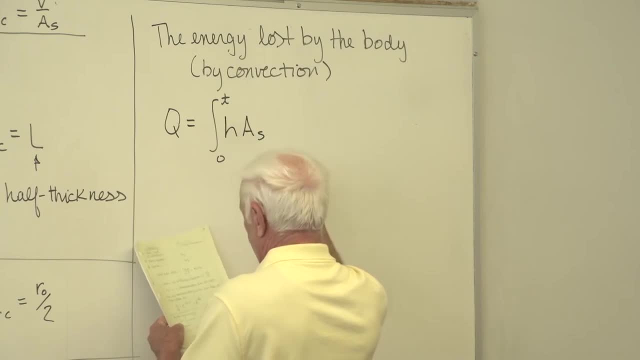 pardon me, HAS. and then we have our Theta d time, Convection by convection. Here's convection, Newton's law, HA, Delta T Theta is Delta, T, T minus T, infinity DT, time, integrate with respect to time. 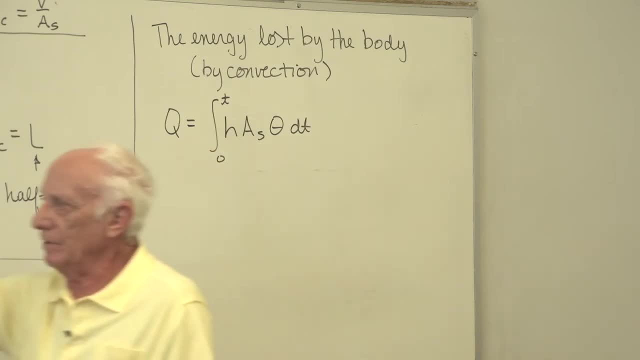 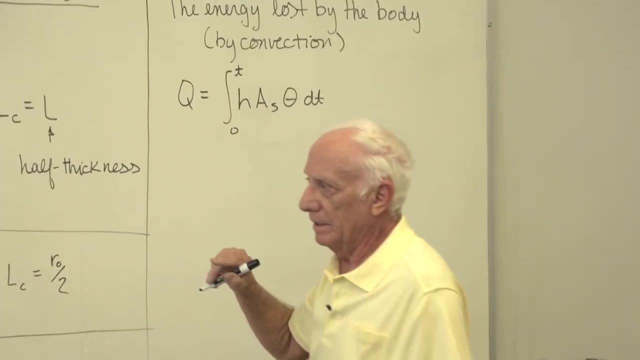 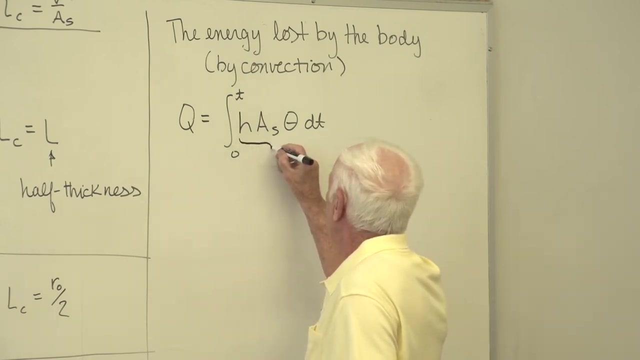 Where you see Theta in here. put the boxed equation right there, Put that right there into there and integrate the exponential function. Just so you know the Newton's law, HA, Delta, T is in watts. A watt is a joule per second. 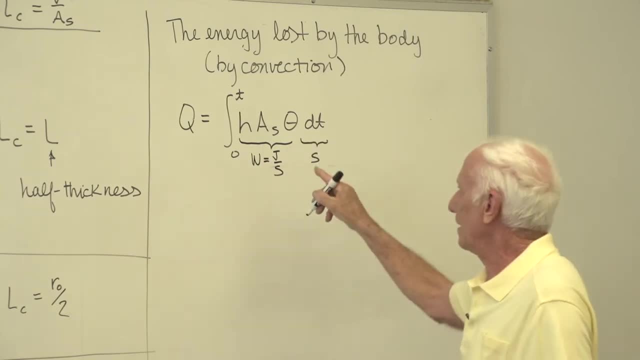 What's this guy here? Seconds. When I multiply joules per second times seconds, I get joules Capital, Q is joules Little, q is watts, Q in joules is energy And, of course, watts is the heat transfer. 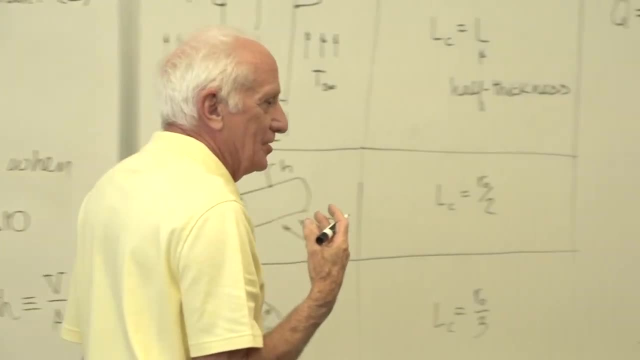 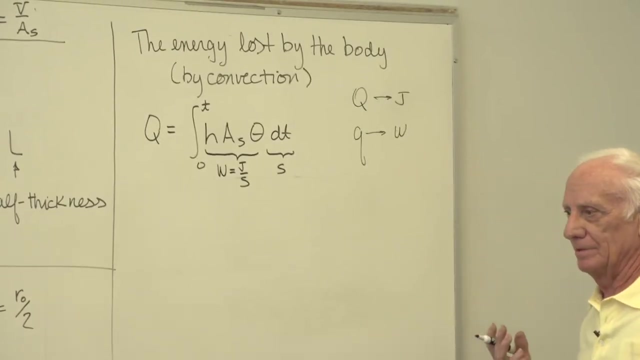 the power watts. So now we've got two q's: a capital Q and a lowercase q. You talk about energy. you talk about capital Q. You talk about heat transfer. you talk about little q. Okay, put those guys in there. 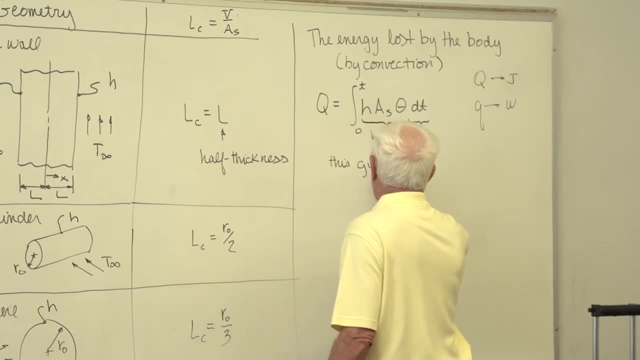 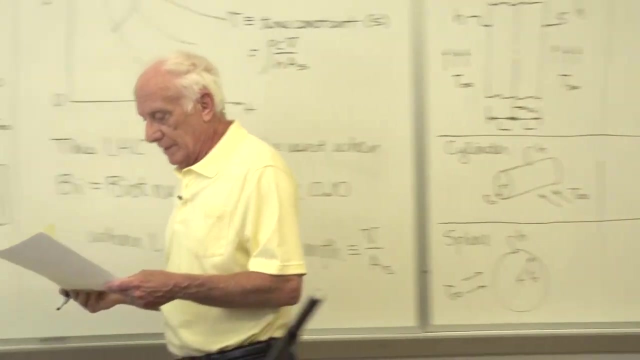 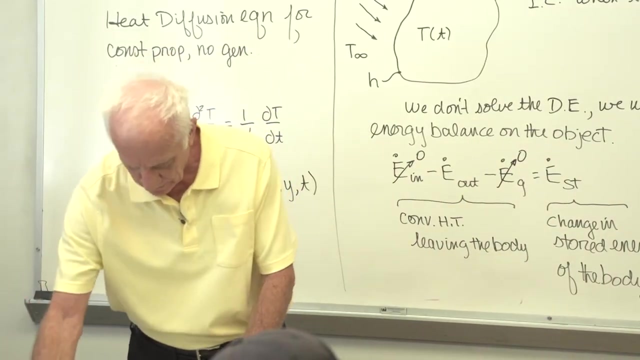 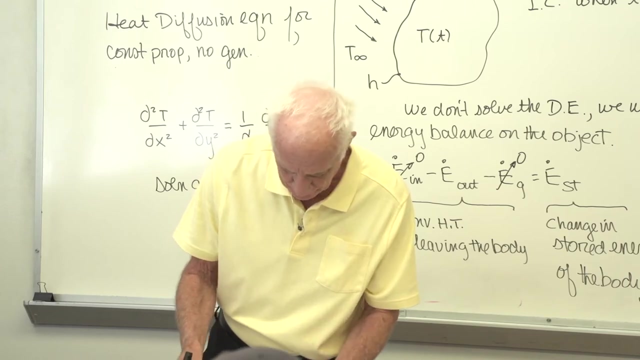 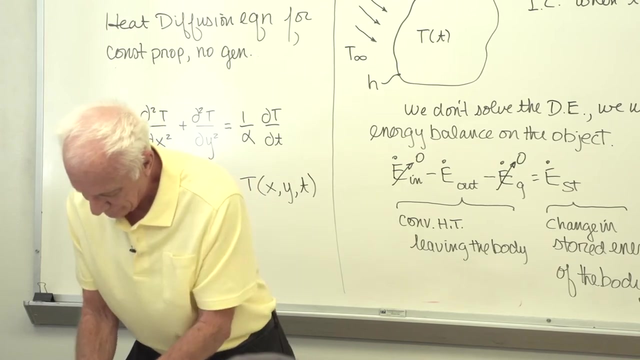 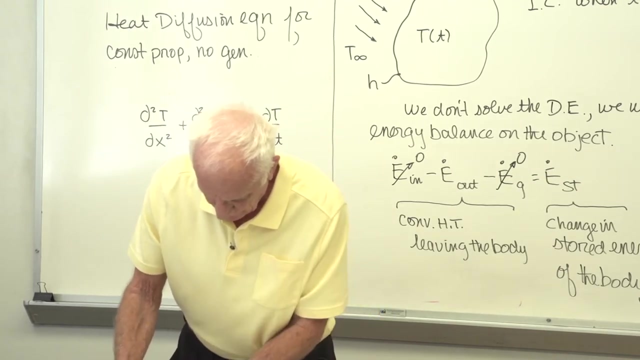 do the integration, I get q. So there are the two equations that we need to solve. Okay, so let's see what I got here. Any questions before we go on then? Okay, Well, let me think here. Oh, here, it is All right. 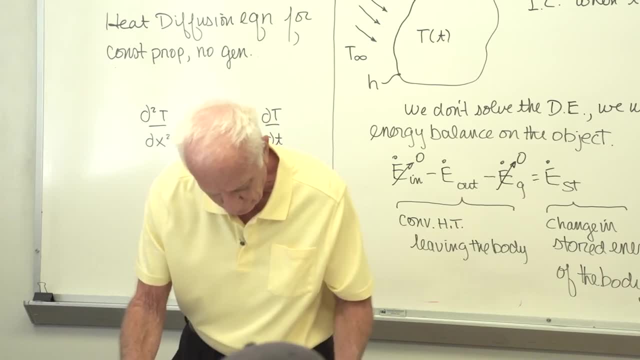 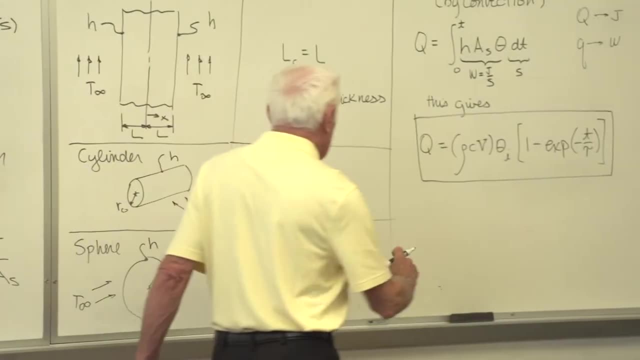 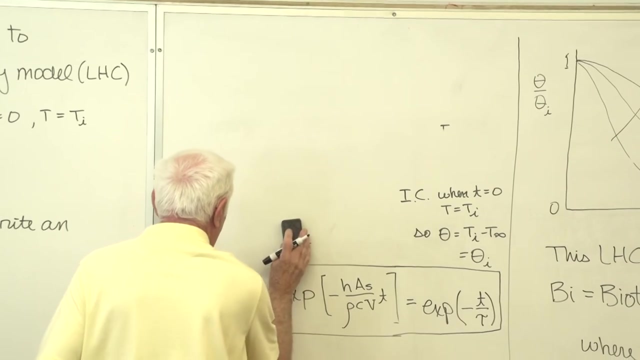 So we're going to then take an example. The example that I'm going to work is a copper sphere. Let's put that on the middle here. So we're going to look at a copper sphere being cooled by air. I might need him. I'll leave him up here. 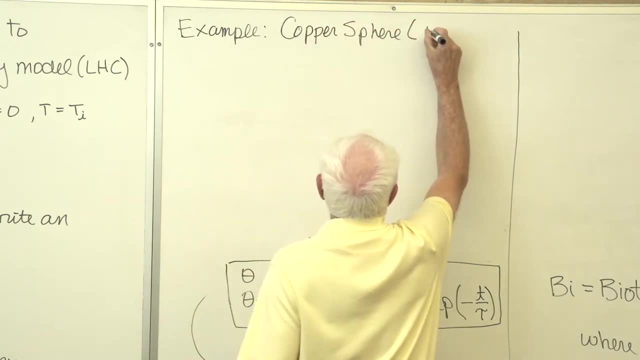 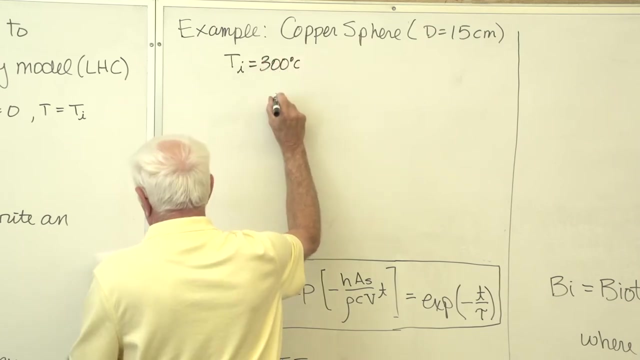 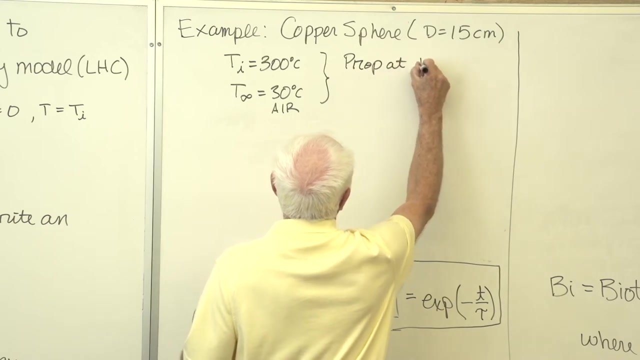 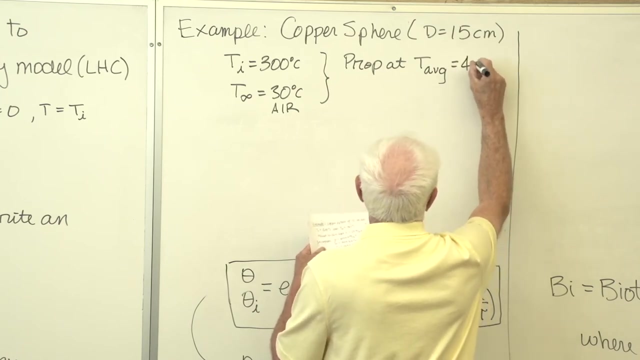 Diameter is 15 centimeters. Yeah, Initial temperature: 300.. Air temperature T infinity: 30 degrees C. Properties At T average. you don't want to take the properties at the starting temperature. You don't know what the final temperature is. 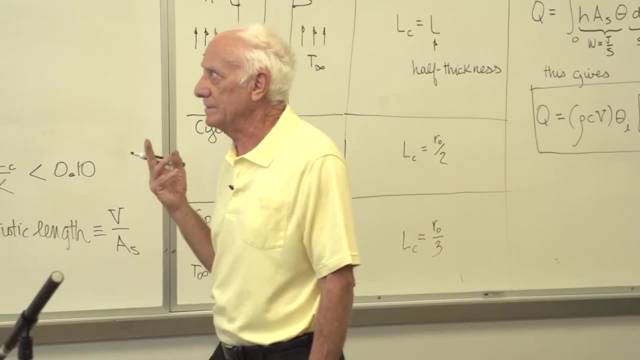 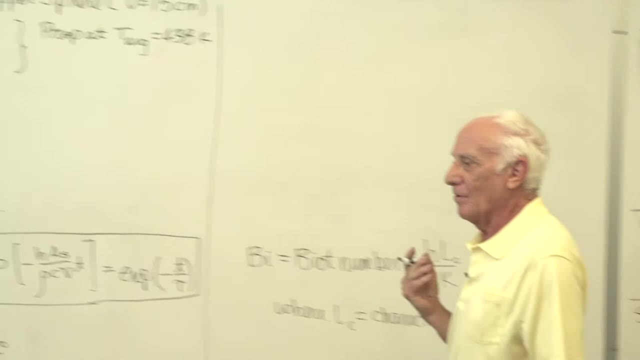 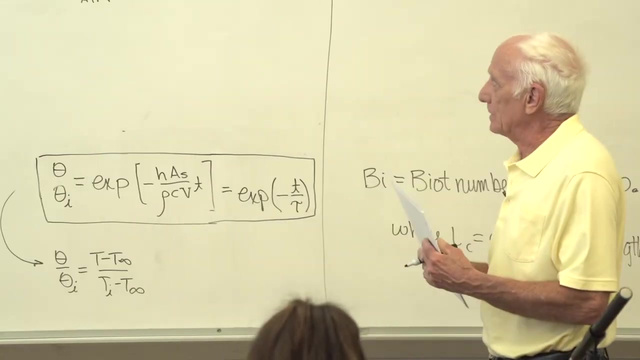 So probably your best guess is to take the properties at the starting temperature- starting temperature plus air temperature- and then take the properties at the starting temperature And once you solve the problem, go back and put the right final temperature in there. I want to know the temperature. 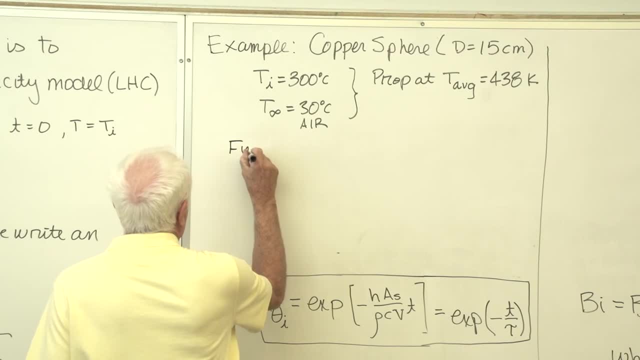 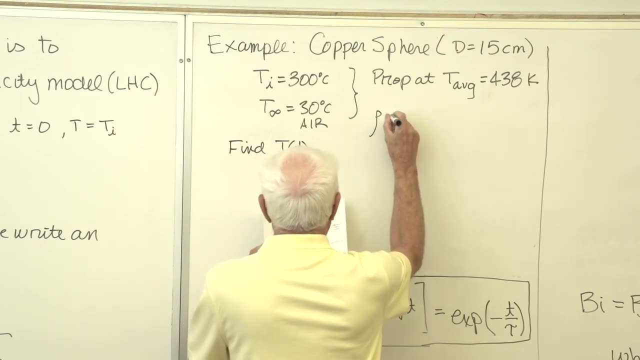 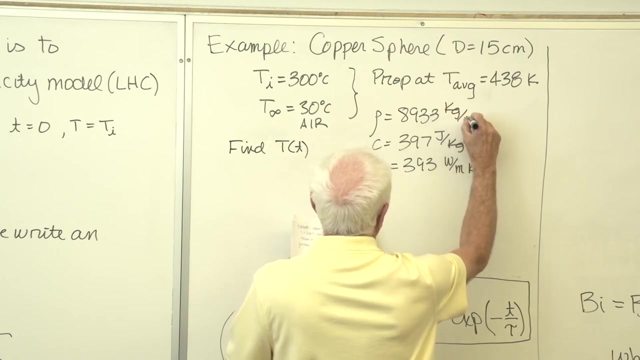 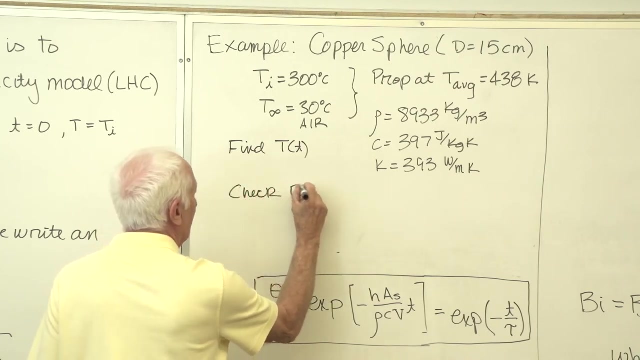 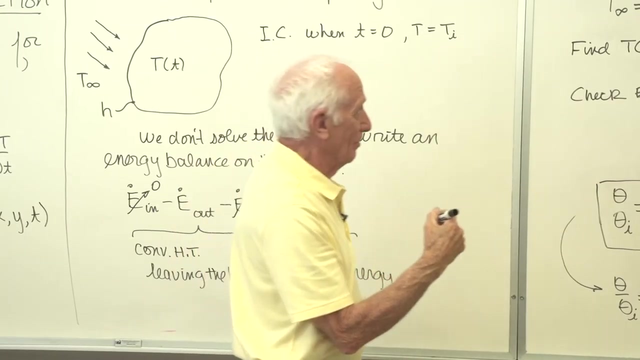 how the temperature varies with time. So find T as a function of time. I'll put the properties down for copper, Step 1, Chapter 5.. Check Bo. Maybe you get lucky and the Bo is less than one-tenth and you can use this model, the simple model. 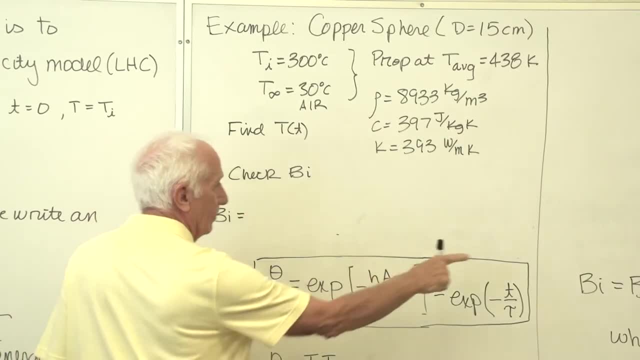 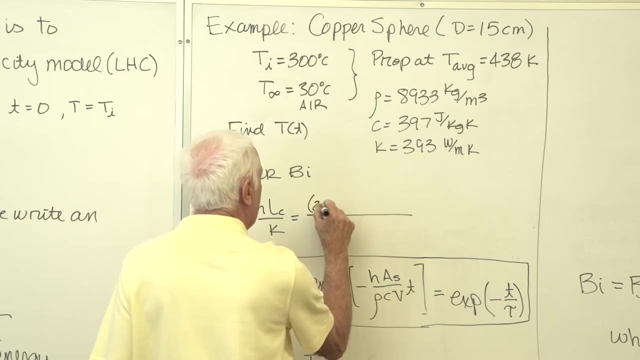 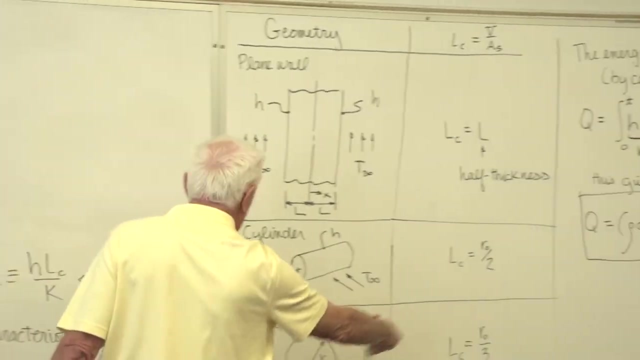 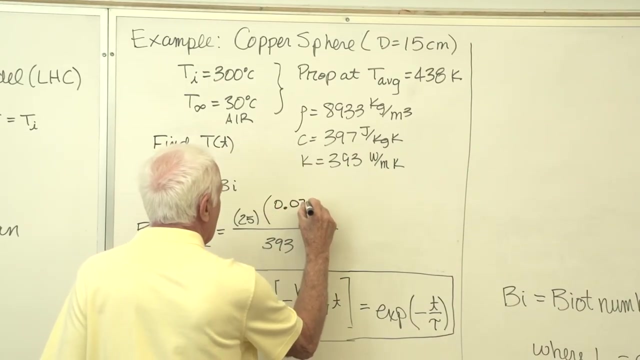 Okay, Bo, equal HLC over K, H 25, K 393, L sub C. from the table geometry a sphere, L sub C, one-third the radius. the radius is seven and a half, 0.20 is 159, which is. 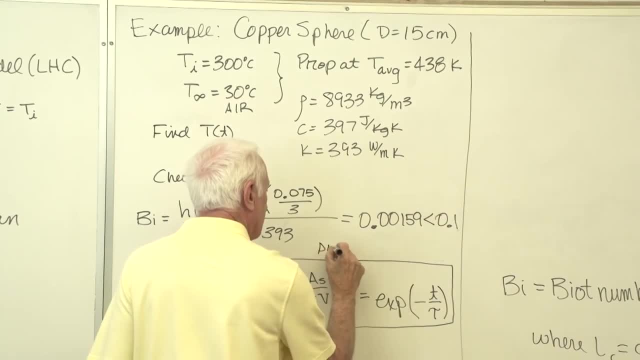 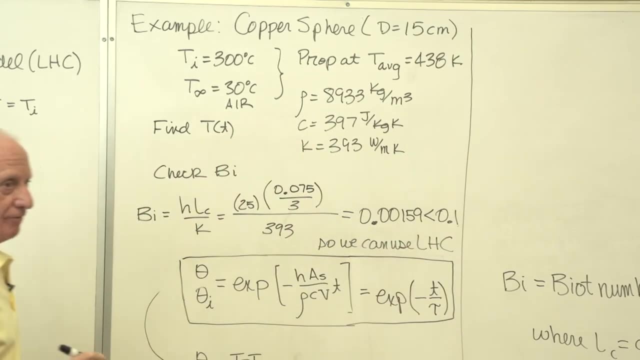 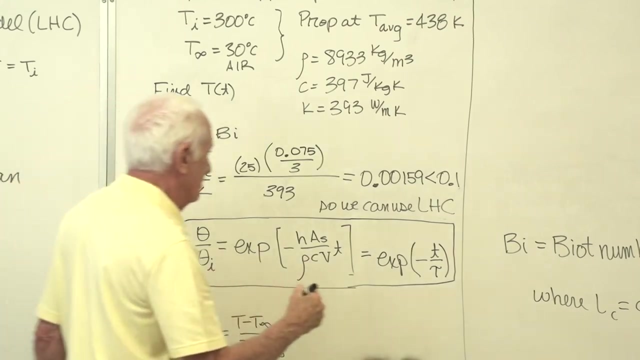 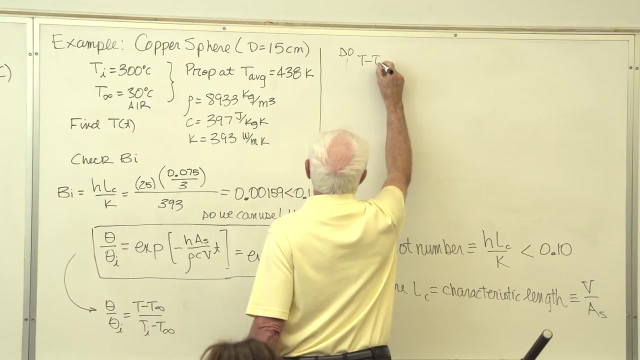 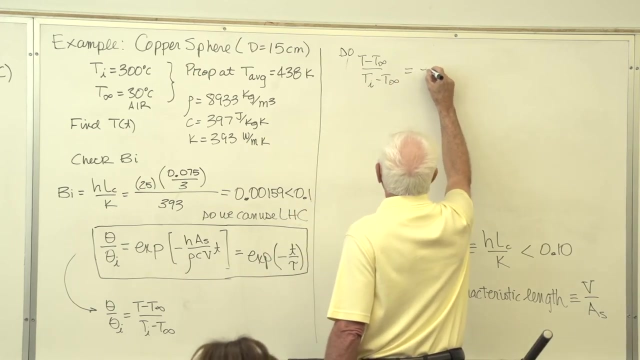 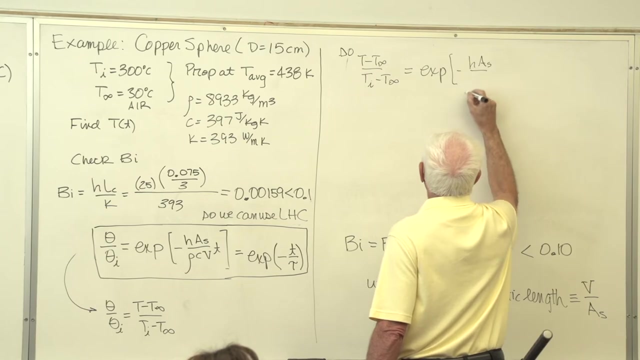 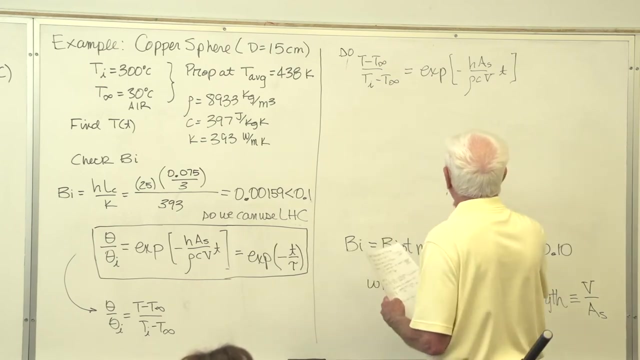 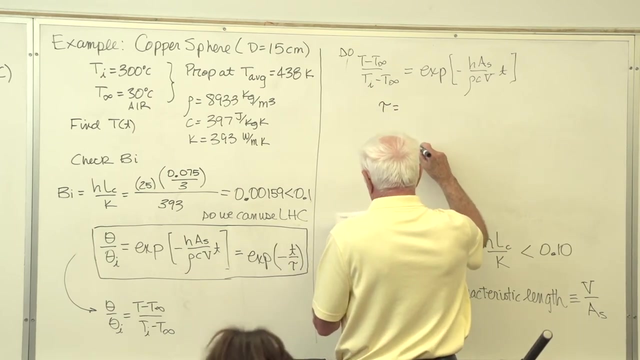 a lot less than one-tenth, so we can use lumped heat capacity. First decision done, I get the easy way out this time. Here's the equation in the box. Here's the equation If I want to find the time constant. tau, my time constant, row C. 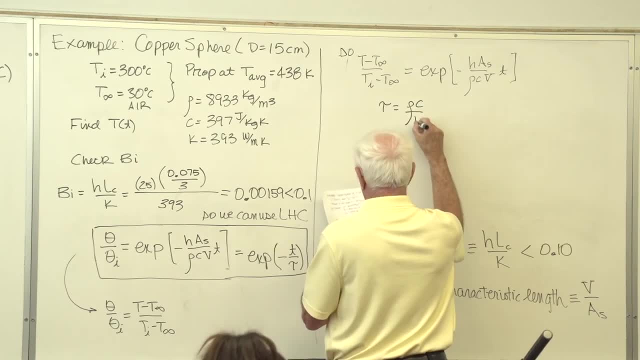 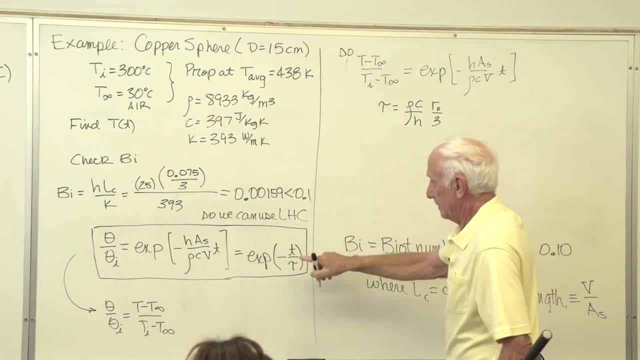 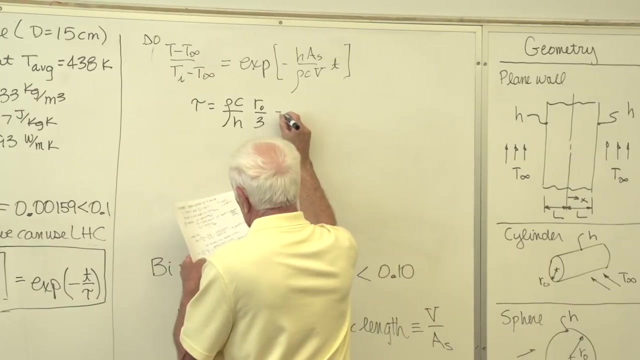 H over C over H are not over 3, L sub C, V over AS is L sub C. Put those numbers in there I get 35.38,, 35.38,, 35.38,, 35.38,. 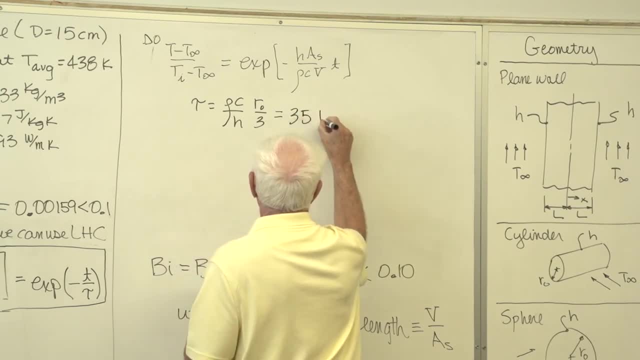 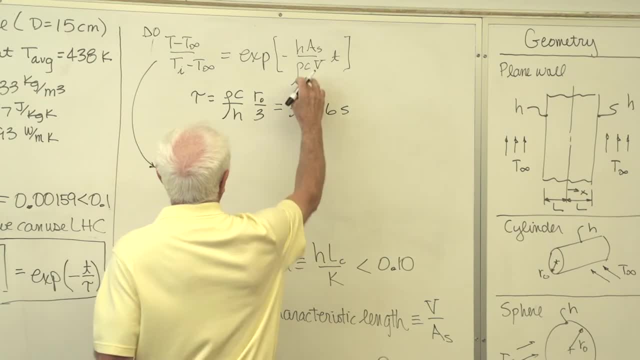 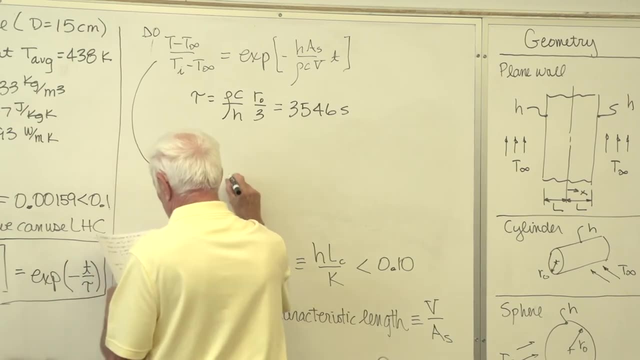 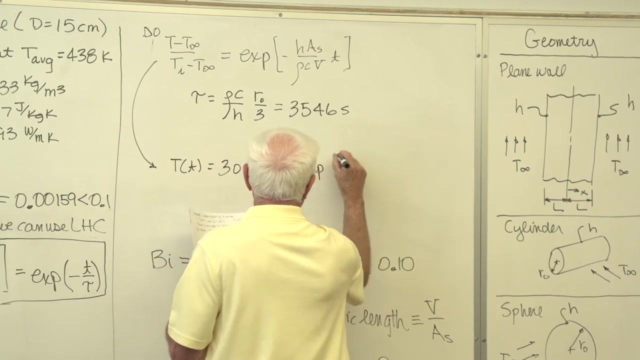 So then I know everything here: the properties, I know h, I know t, infinity, I know ti. So t as a function of t, then when you put the numbers in T, put t in in seconds and the time will come out to be degrees c. 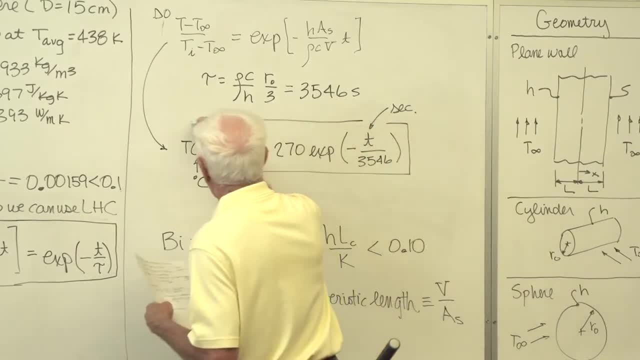 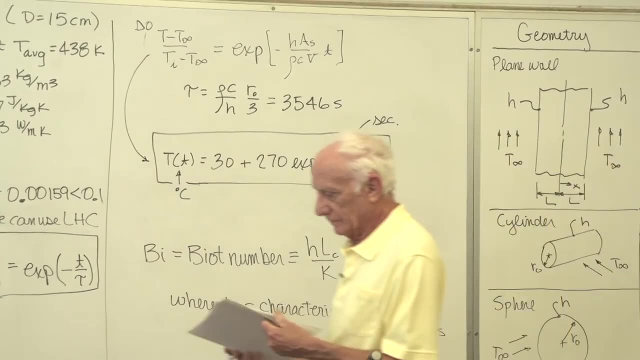 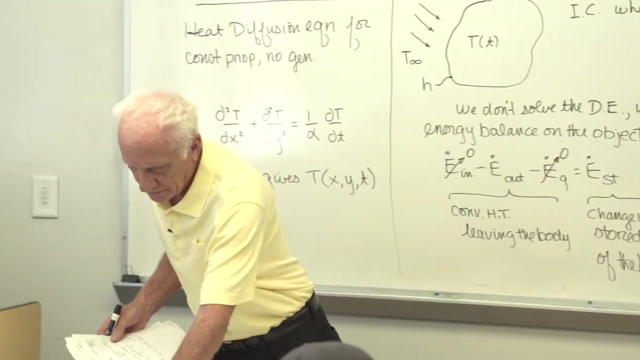 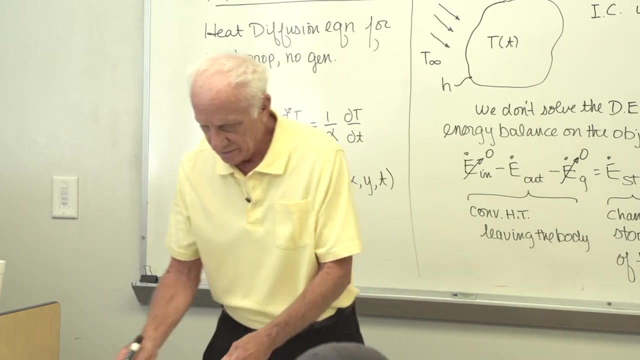 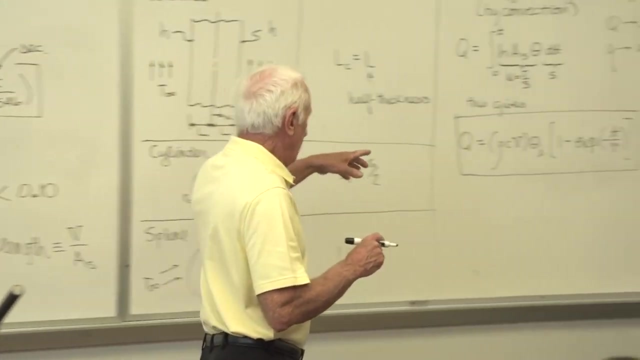 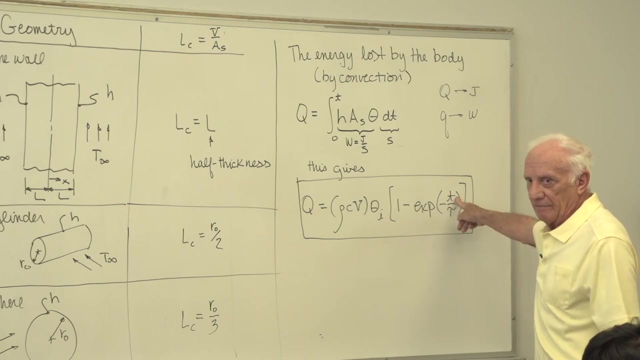 So that's my solution. then Now, if somebody asks me, by the way, how much energy is lost by the copper sphere, I say, okay, here's over here The first five minutes: 60 seconds per minute times 5,. 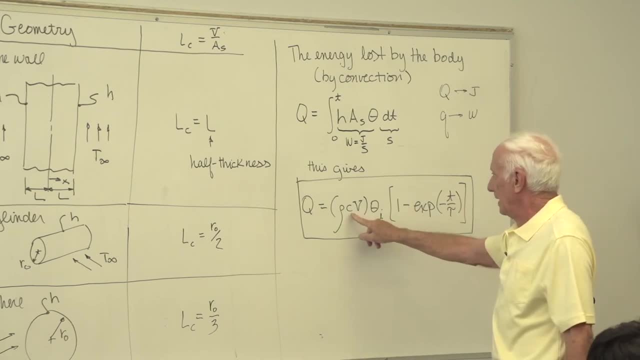 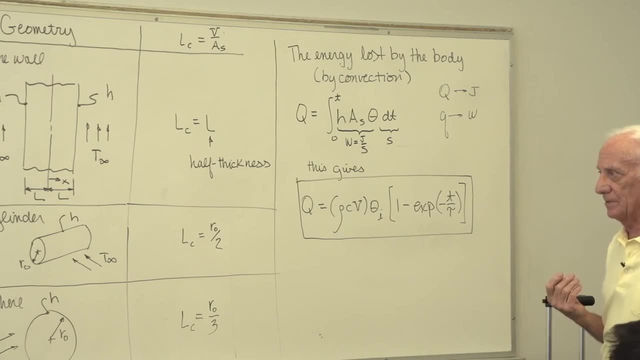 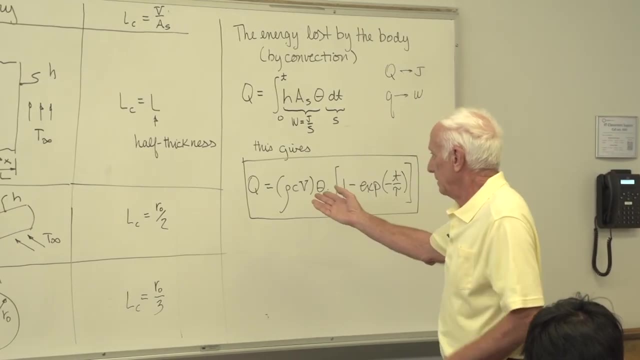 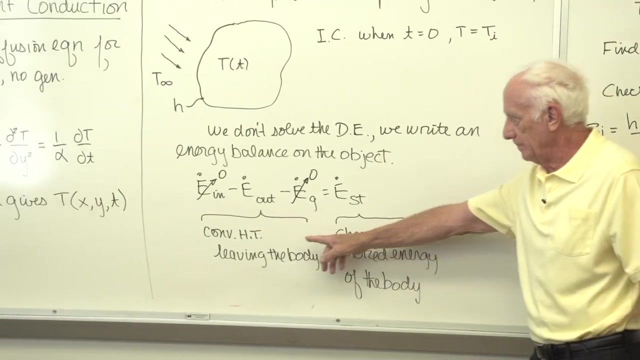 Now you say: well, how much heat transfer has occurred, How much energy has gone out by convection? It's the same answer. The change in internal energy is the same as the amount of energy lost by convection. says it right here. 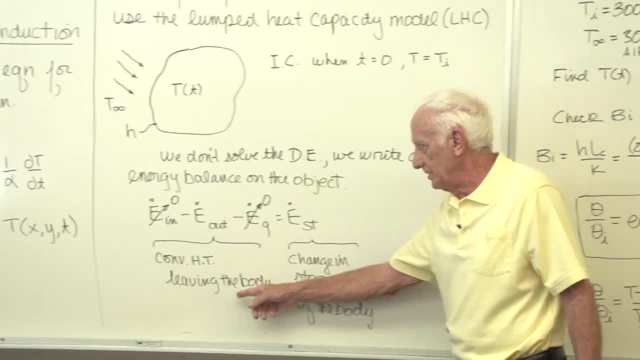 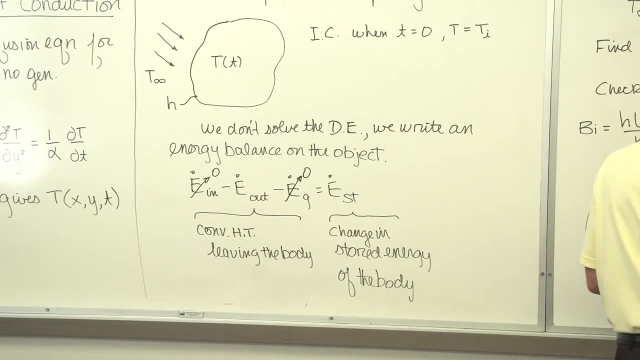 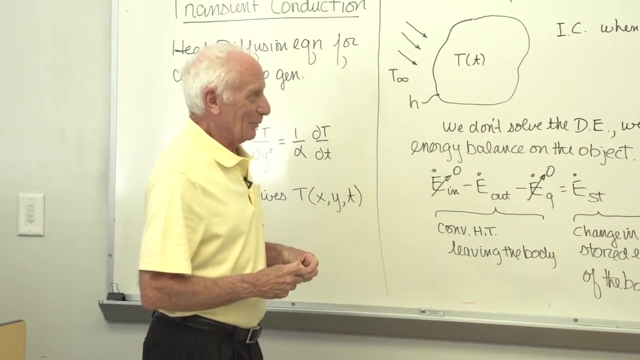 Change in storage is the same as how much energy goes out of the body by convection. Okay, All right. Any questions on that, then? Okay, So now, of course, the obvious question is: yeah, but what if the B0 is greater than 110?? 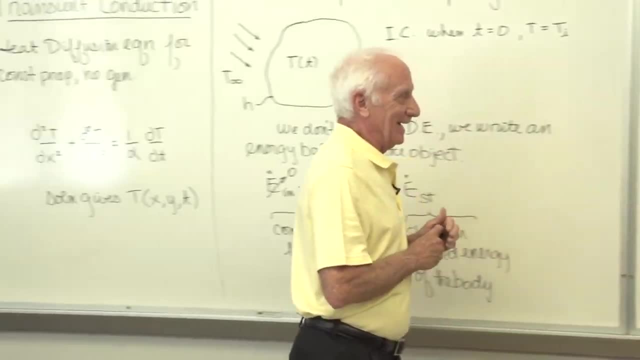 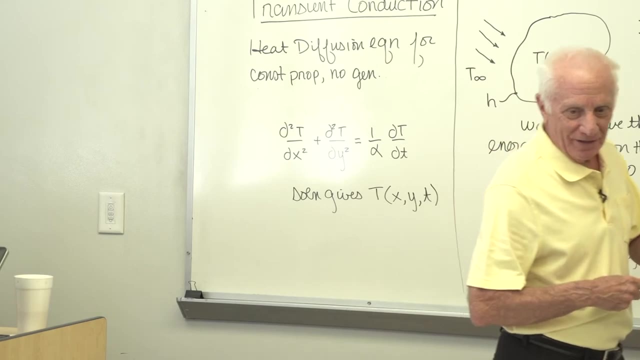 Okay, Now we got much more difficulty mathematically. Yeah, That's going to be Monday. We'll save that for Monday, Okay, All right. So I want to go over some things about the midterm on Friday with you, So let's do that right now. 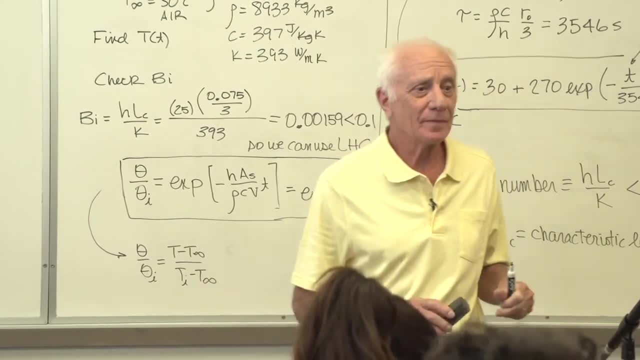 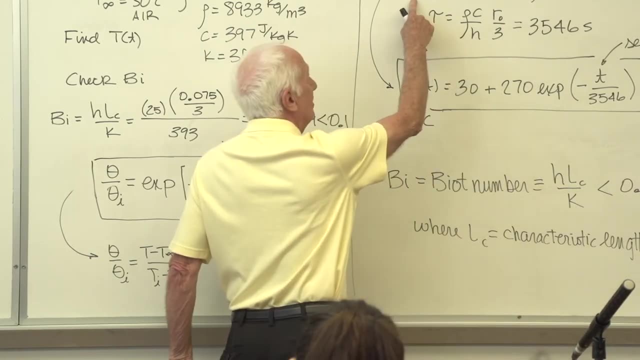 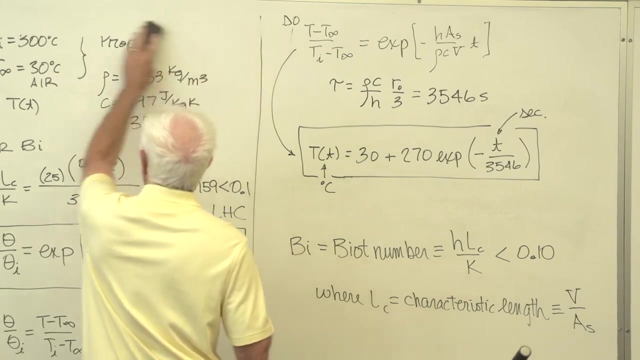 Any questions before I erase any of this. Yes, Which one now here? Oh yeah, It's this guy here: 300 minus 30.. All right, Let's take a look then. a little bit of review and it's going to. 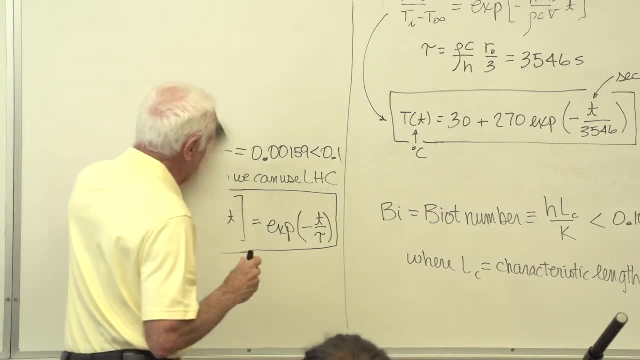 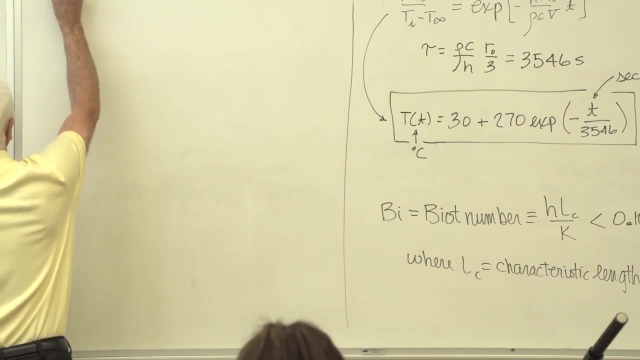 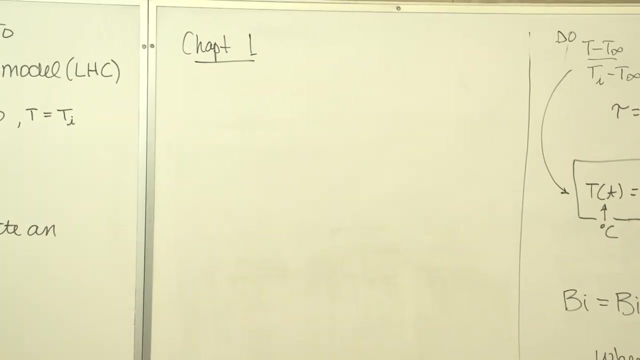 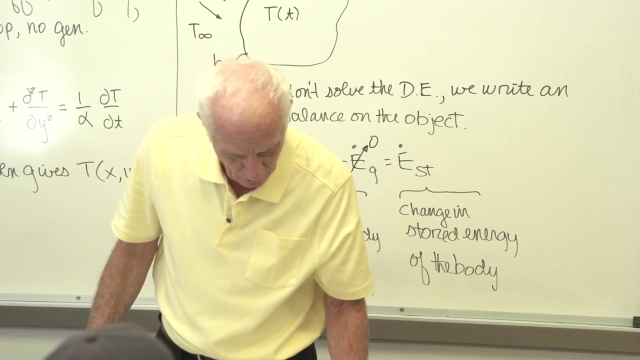 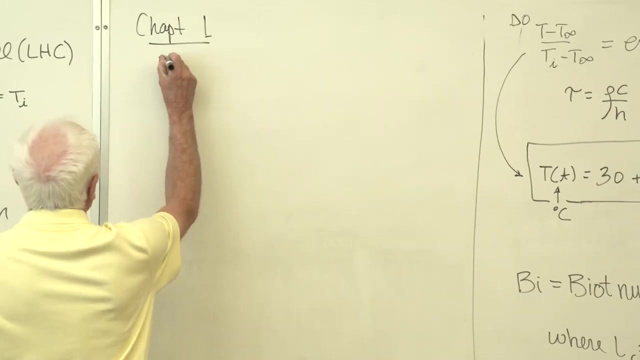 be not in great detail, but just to jog your memory of what could occur on the first midterm. So here we have Chapter 1.. Is Elizabeth here, I guess up front? here we're done a paper for you. Let's take a look and see Chapter 1, Fourier's Law. 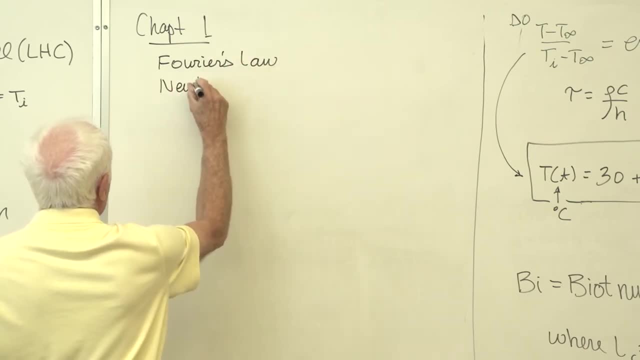 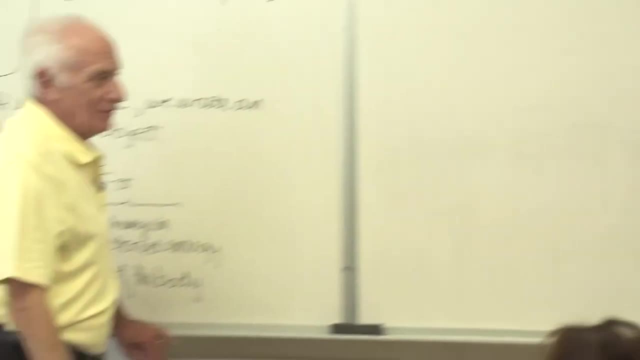 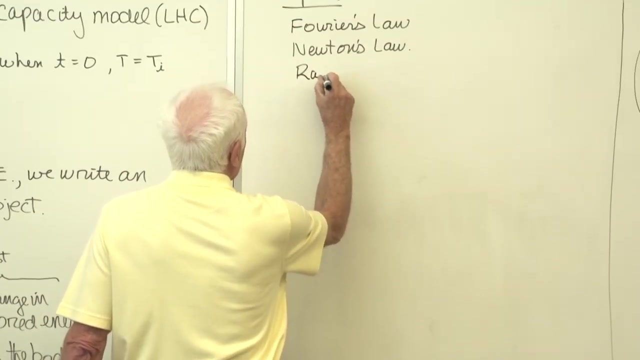 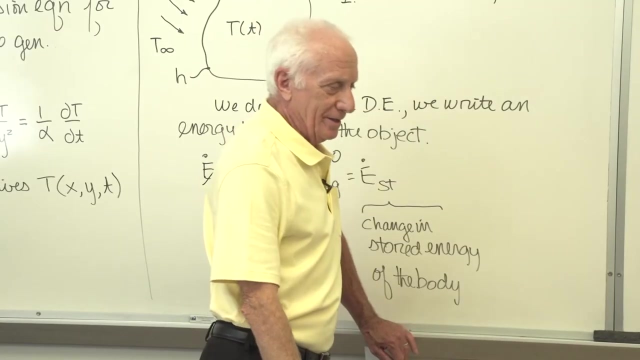 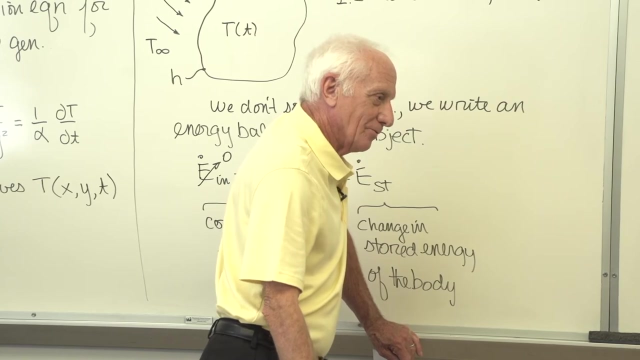 Newton's Law convection: Yes, Yes, Yes, Yes, Yes. Fourier's law: kA over L Delta t. Newton's law: HAs: Delta t Radiation: small object in a large surroundings. Epsilon sigma A: t object to the fourth. 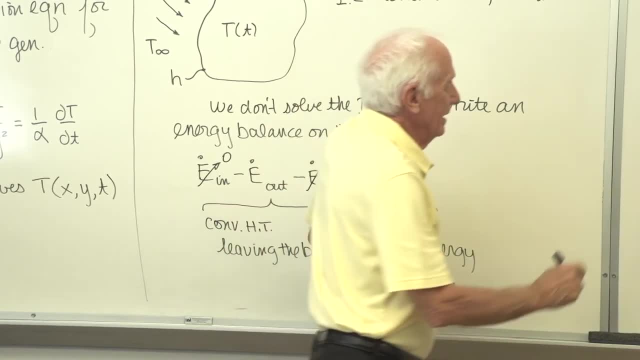 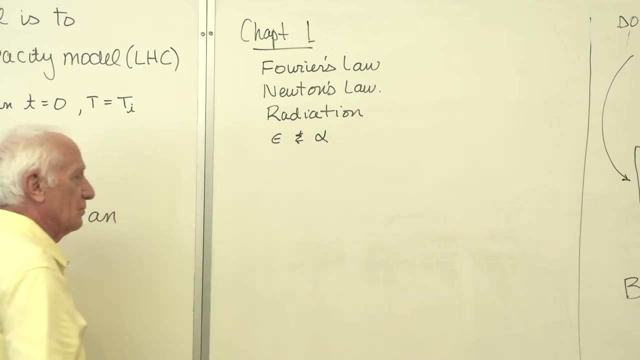 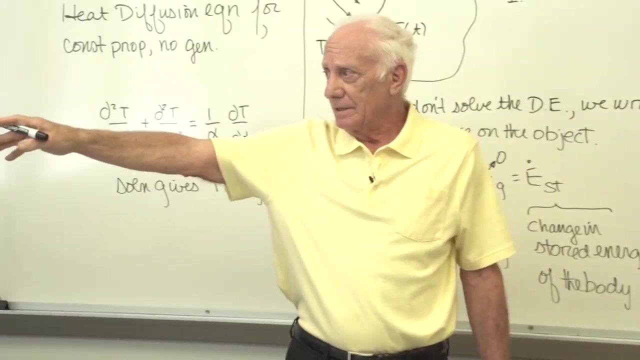 minus t surroundings to the fourth, That's for a black body. epsilon is one alpha, that's emissivity is one, The absorptivity alpha. if you multiply, like the solar input on the street out there, times alpha of black asphalt. 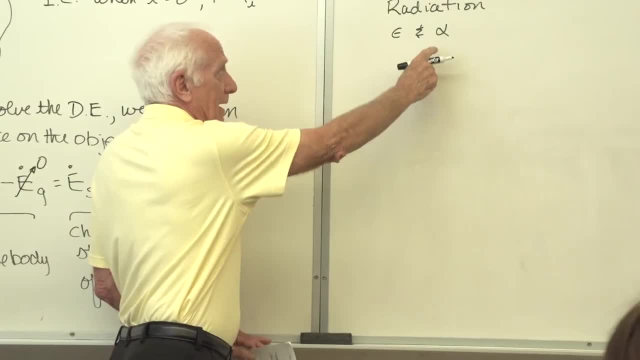 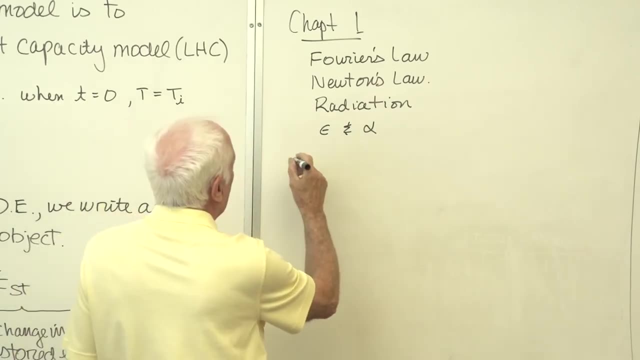 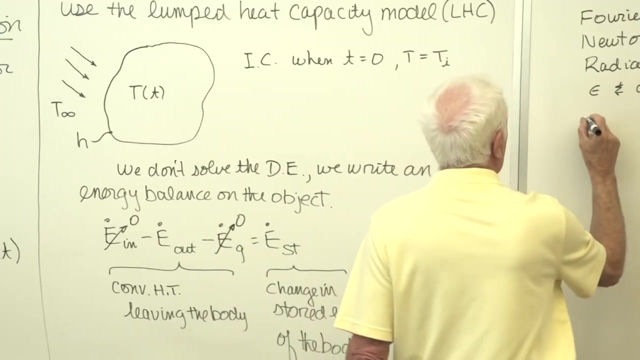 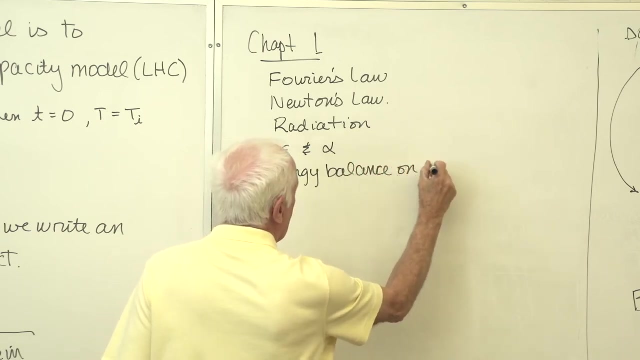 then that's how much is absorbed by the black asphalt: Alpha is the absorptivity, epsilon is the emissivity. Then we had like over here, energy balance on a control volume, Then we had a surface energy balance and that gets us to Chapter 2.. 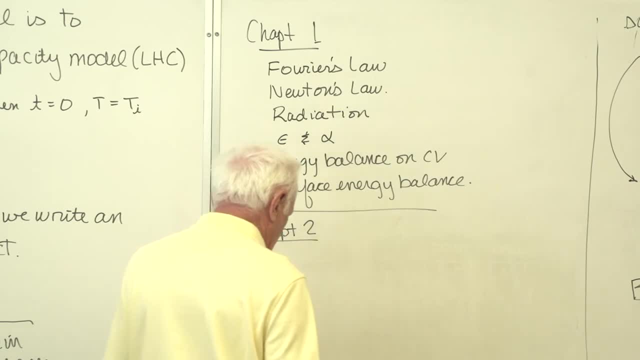 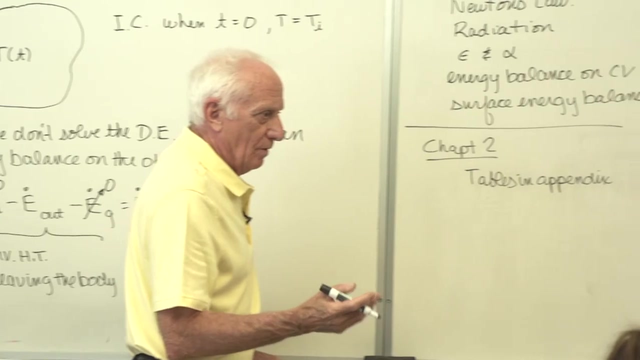 Chapter 2, real short, but Chapter 2 starts out with the tables in the back. Just to become familiar with what's there for you, What was the solid, What was the liquid, What was the gas, At what temperature? All that stuff is in the tables. 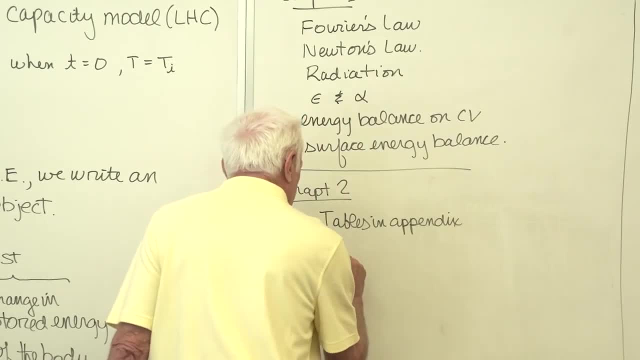 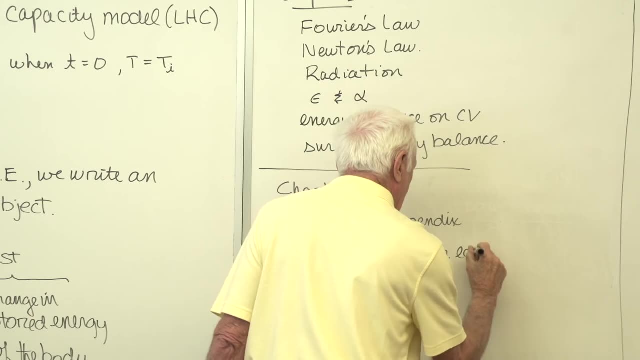 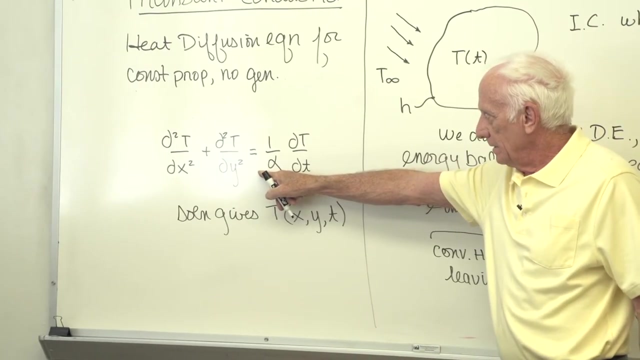 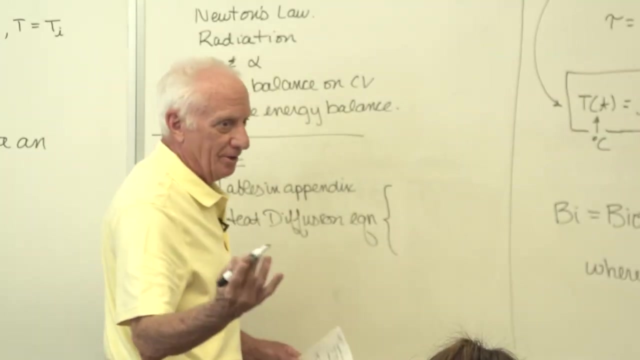 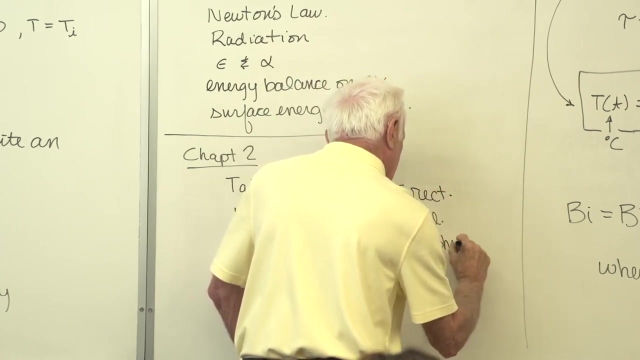 When then? heat diffusion equation: Different versions. The rectangular version- There's one of them right there. That's the heat diffusion equation for constant properties, no generation, So obviously that should be on your equation sheets. Rectangular, cylindrical, spherical. 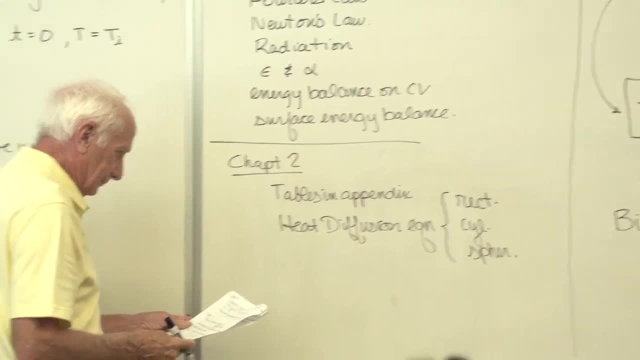 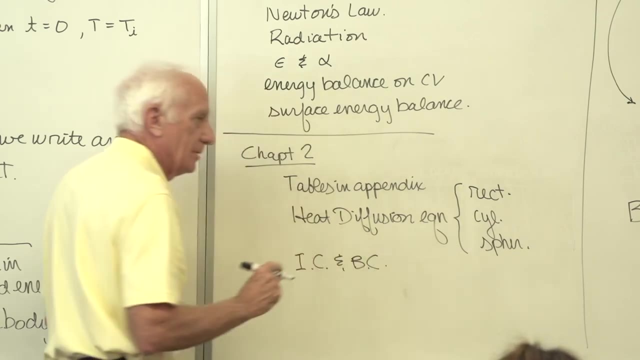 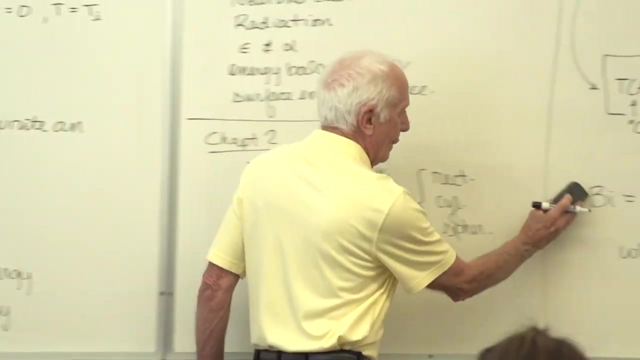 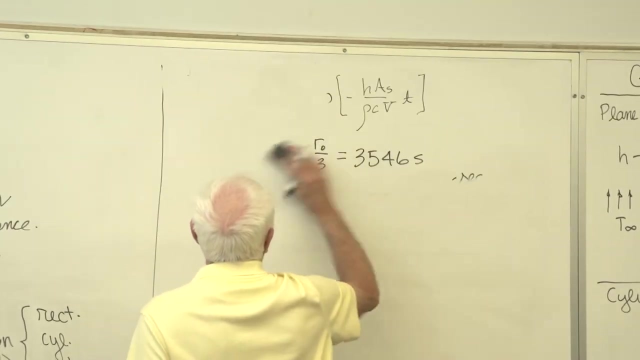 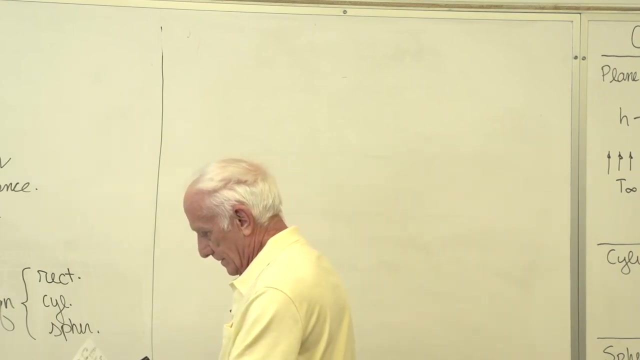 Three equations, Know how to specify initial conditions and boundary conditions to apply to the partial or ordinary differential equation. Okay, That's Chapter 2.. Let's go to Chapter 3.. Okay, Chapter 3 is our resistances. Yeah, All right, We have conduction resistances. 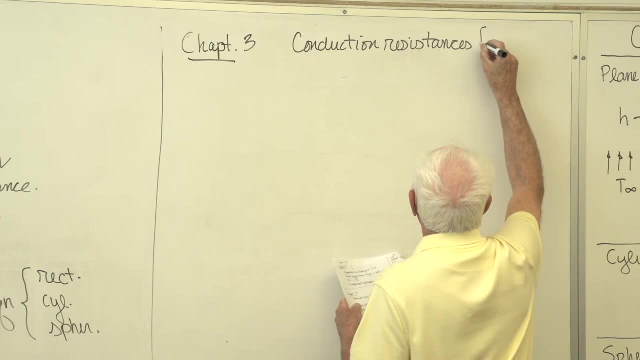 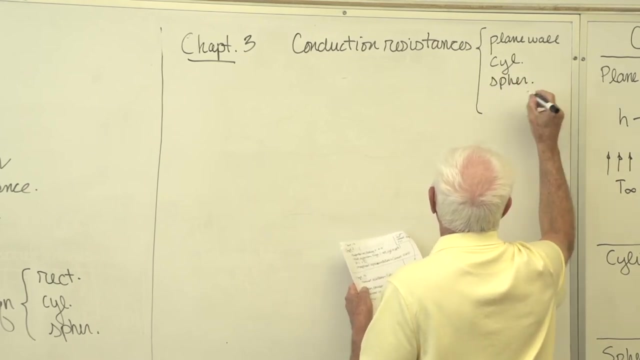 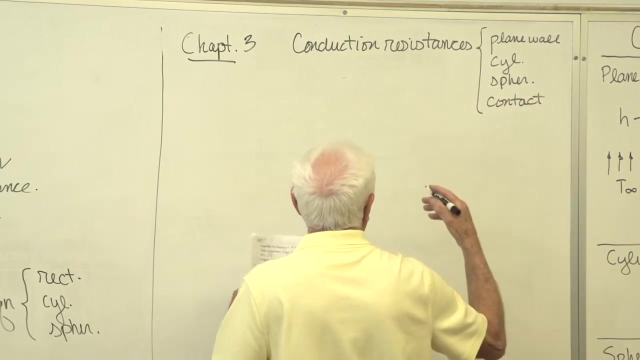 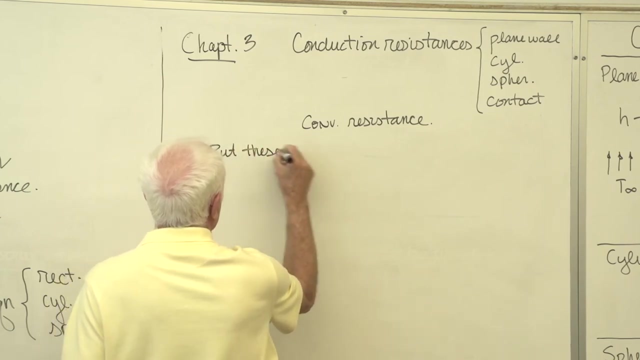 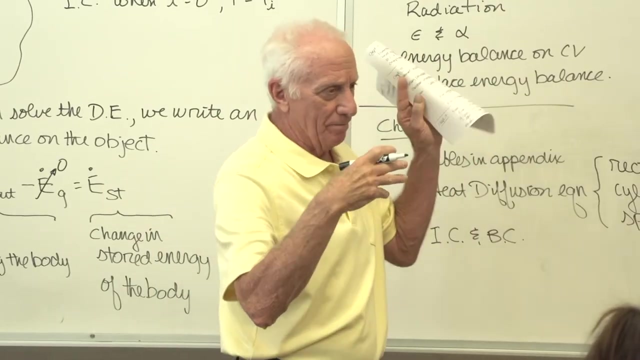 Again, we have plane wall, cylindrical, spherical, and we have contact resistance. Then we have convection resistance. Okay, We have convection resistance, We have convection resistance. Then we put these in series, parallel or others. It's split and some went down and some went up. 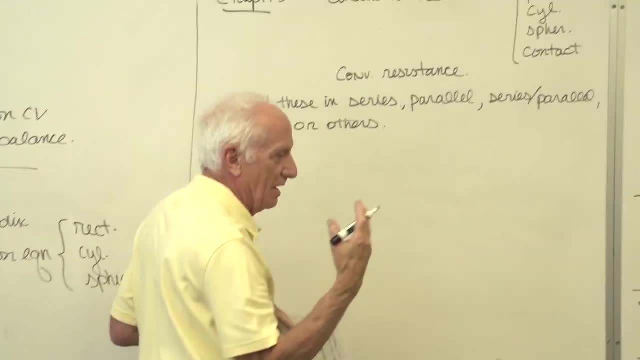 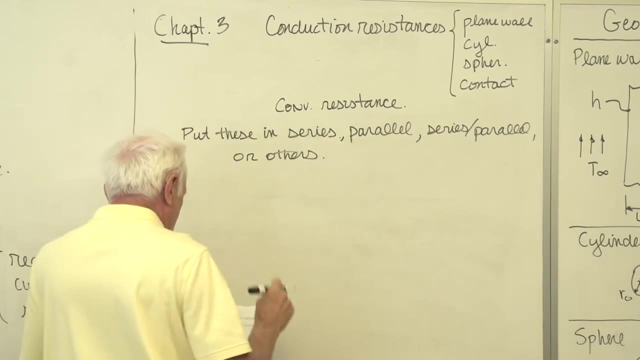 So that's neither of these three. So there's other geometries that you construct these circuits. Fins Possibly use Table 3.4.. Fins of a uniform cross-section area. They give you Qf and it gives you the temperature of. 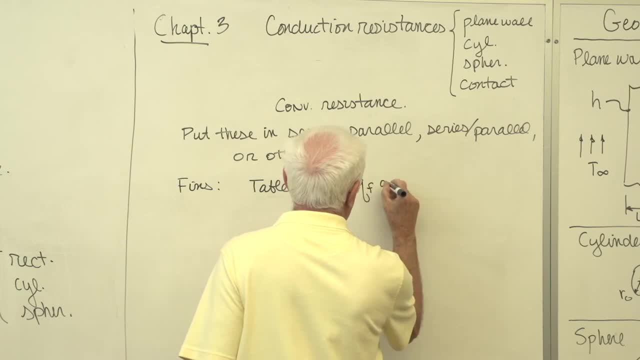 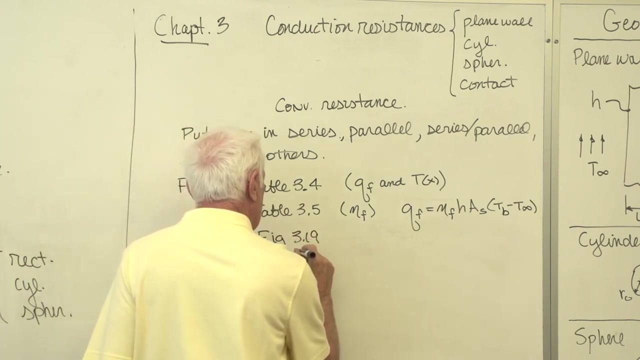 the fin as a function of x. Maybe you can use Table 3.5.. Table 3.5 gives you fin efficiency and then use that to get Qf. But maybe you can use Figure 3.19 or maybe Figure 3.20.. 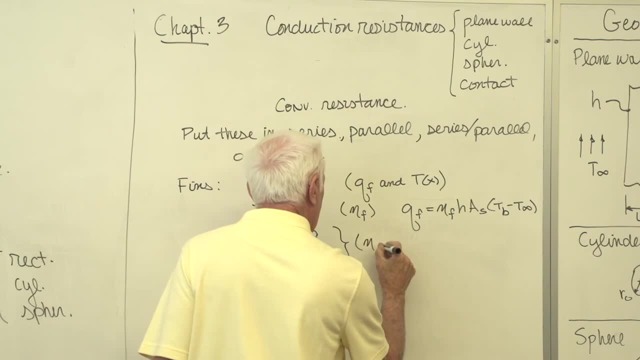 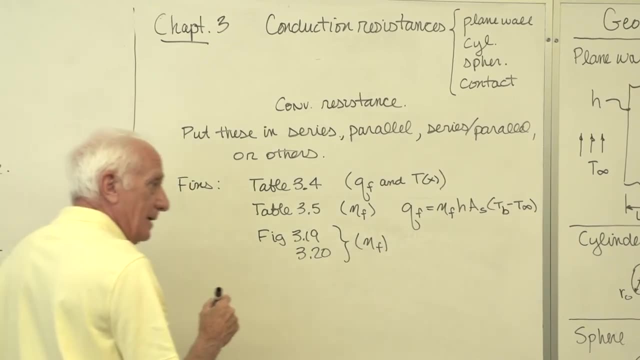 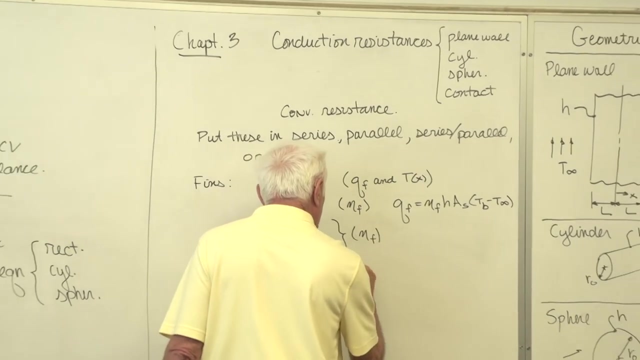 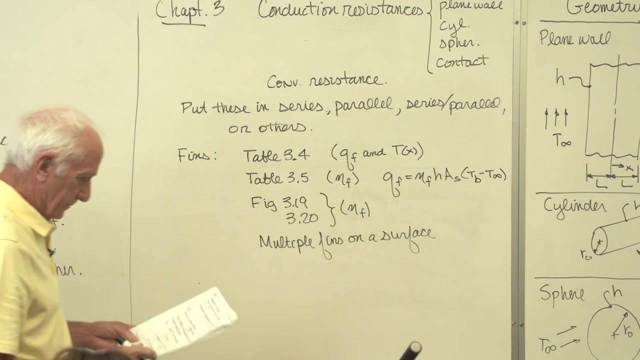 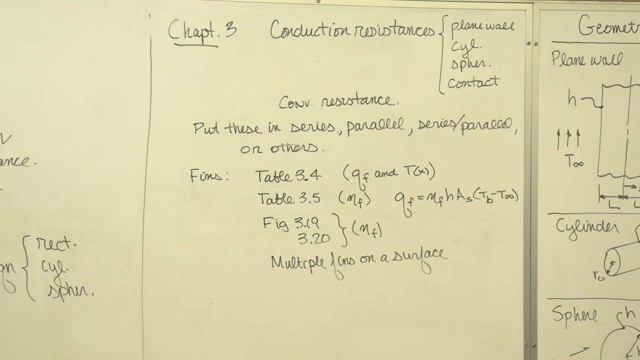 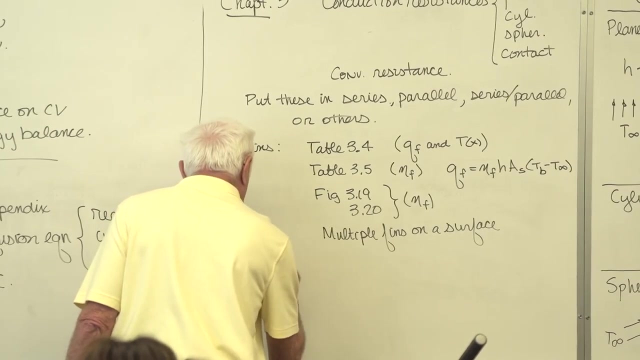 They give you a to f and put it in that equation to get Qf, And then maybe you have multiple fins on a surface. We had problems like that. Now we have Chapter 4, then Chapter 4.. Draw a flux plot. 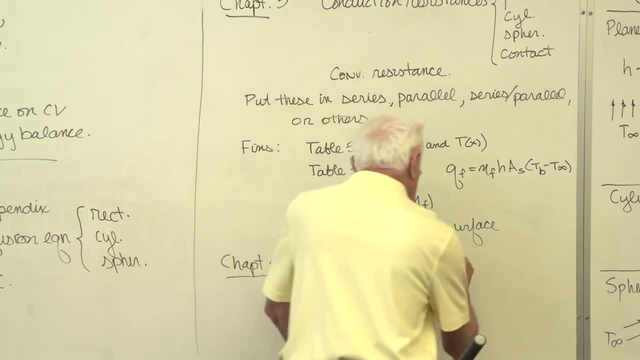 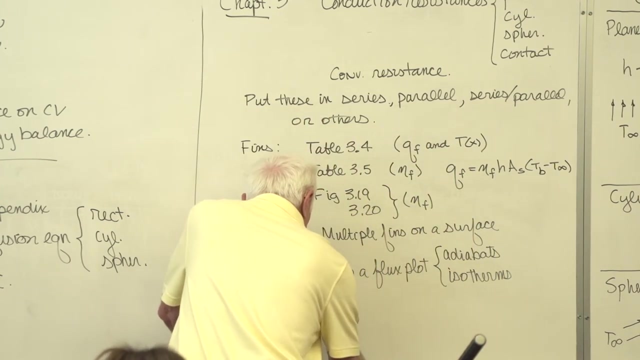 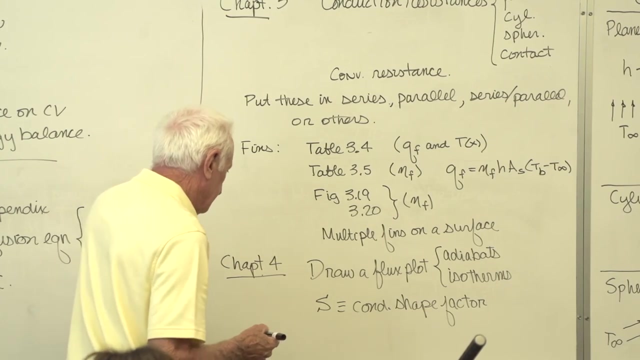 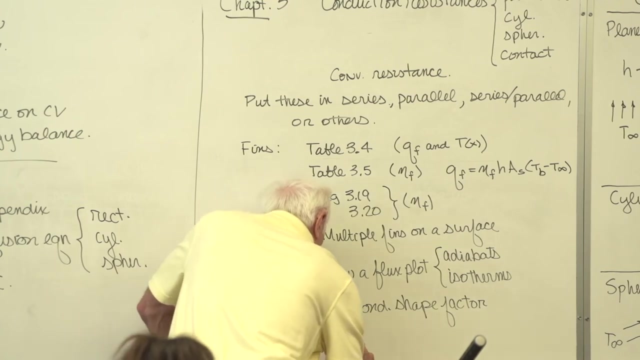 Show the adiabats and the isotherms. Find capital S, Capital S conduction shape factor. Use it to solve for heat transfer. Okay, If you want a resistance, you can use. function if possible. The resistance is 1 over SK. 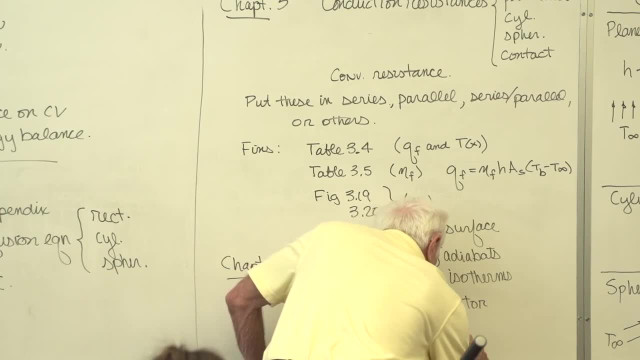 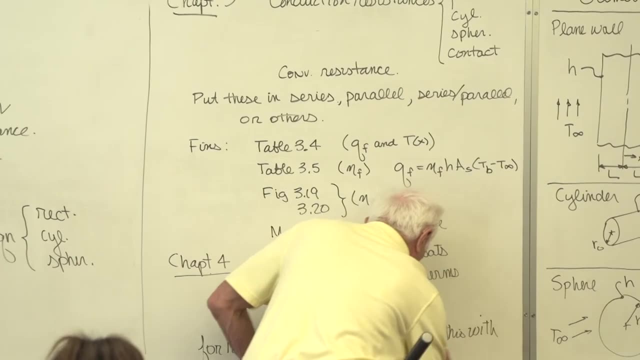 That's going to be 1 over SK x. We're just basing over the speed, But really takeгуild in this掰掰. If you want the 可以 on the Arduino, you're good. You just perform something. 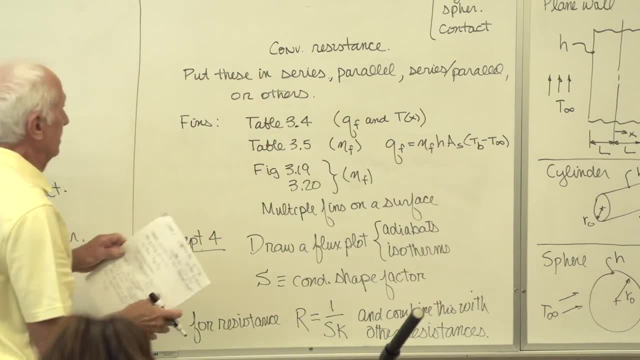 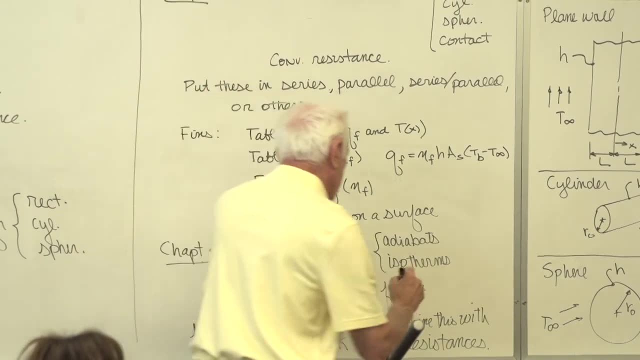 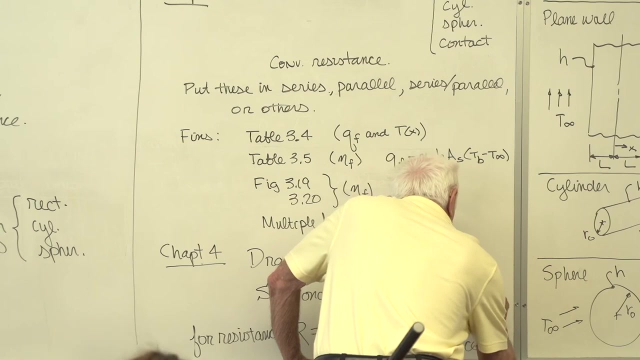 All right, Thanks everybody. you can combine that resistance with other resistances, like the convection resistance, one over H A, S, By the way, this conduction shape factor. then you use Q equal S, K, Delta T. That's how you put S in there to get Q. 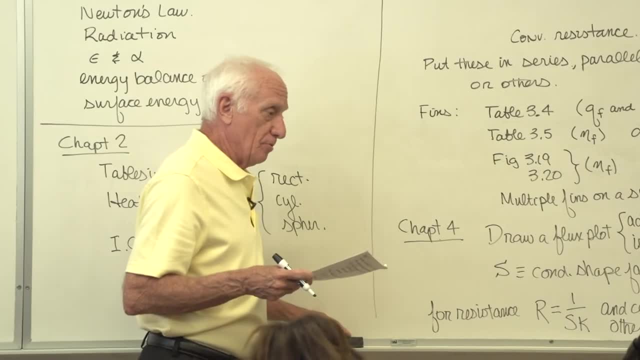 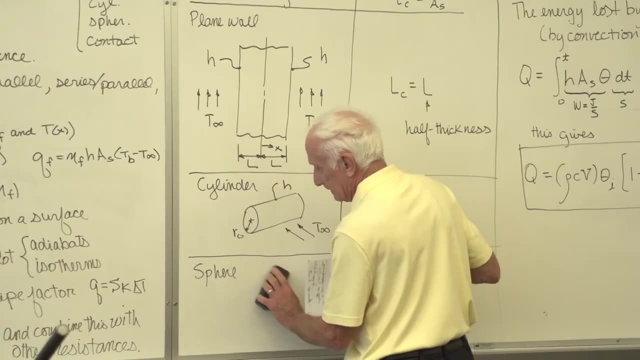 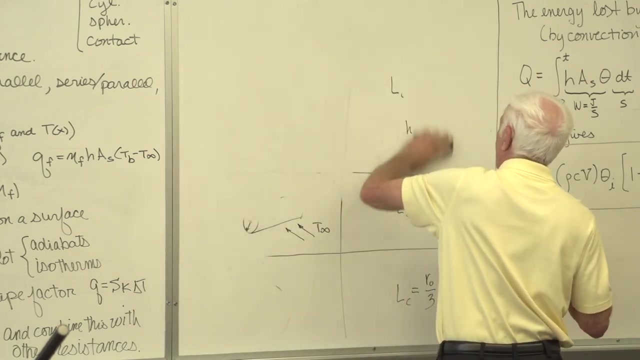 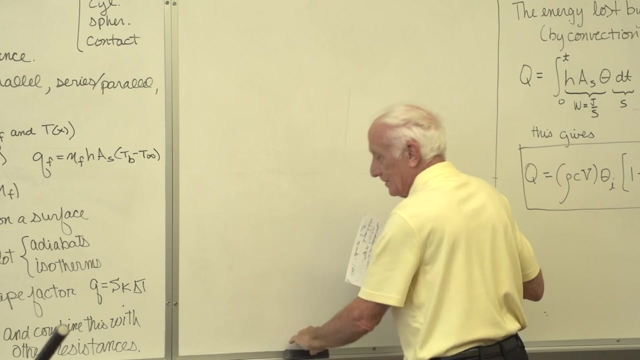 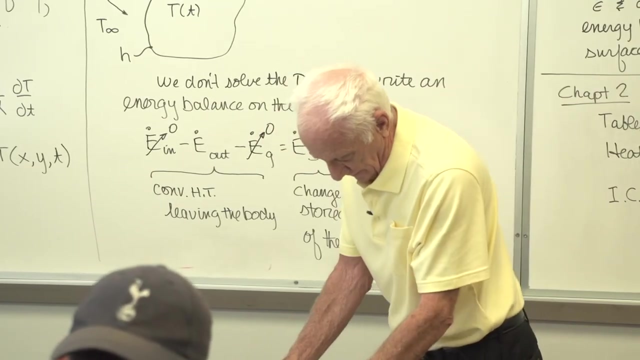 Now the last half of Chapter 4, numerical methods, will not be on the midterm, So stop there. after the conduction, shape factor, capital S. Now let's talk about maybe what you should look at as far as example problems in the textbook. 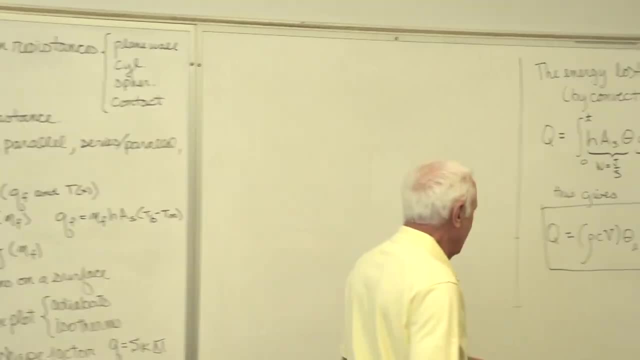 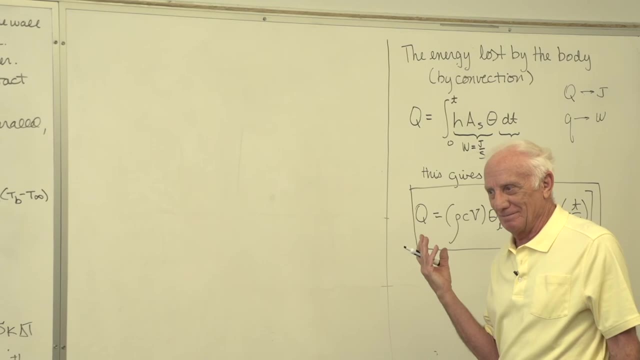 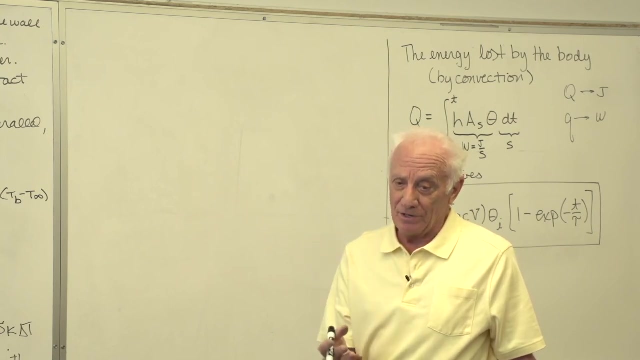 Of course I told you before anything I box in the lecture probably should be on your equation sheet because I think it's an important equation, But beyond that there may be equations or whatever you use to solve homework, If that's important you. 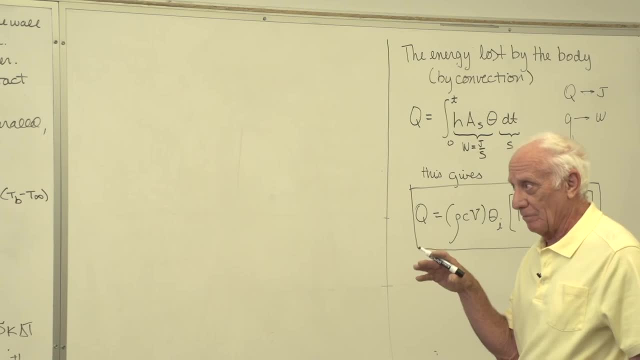 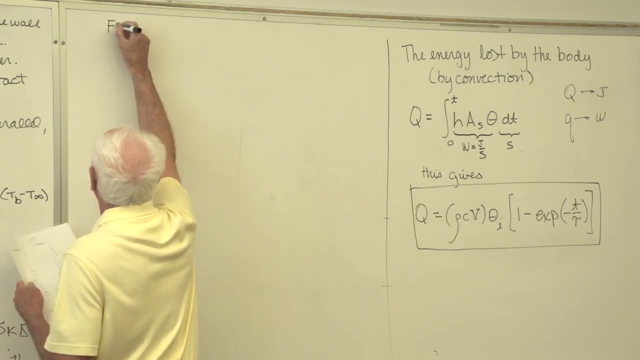 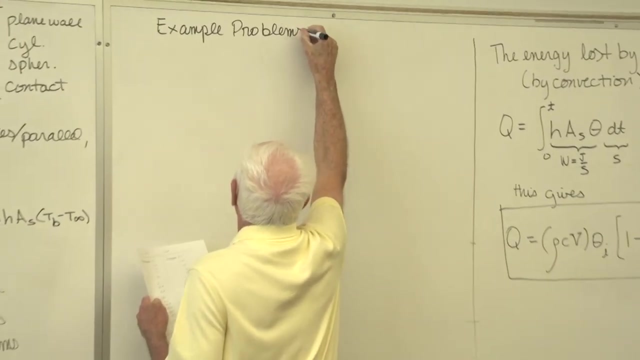 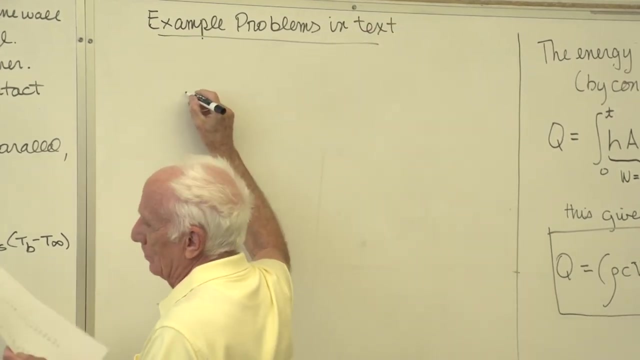 put that on your equation sheet, Not just what I box in class, but what you use to solve homework problems. So here are example problems in the text. It depends what textbook you're looking at, If it's the heat transfer textbook, introduction to heat transfer. 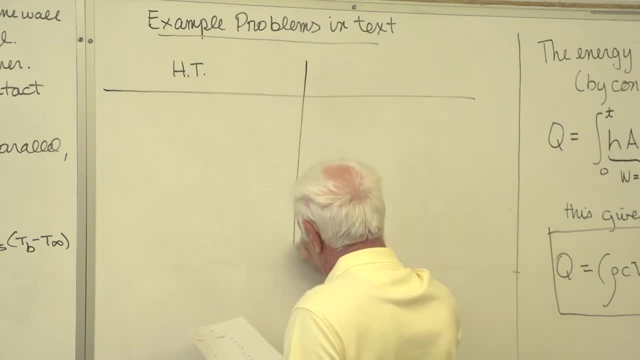 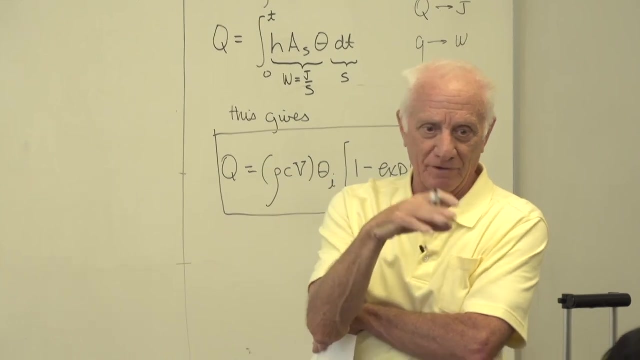 it's going to be the left-hand side. If it's the heat and mass transfer textbook, it might be slightly different. So these are the example problems worked in the chapters in the textbook that I think probably are important for you to look at. 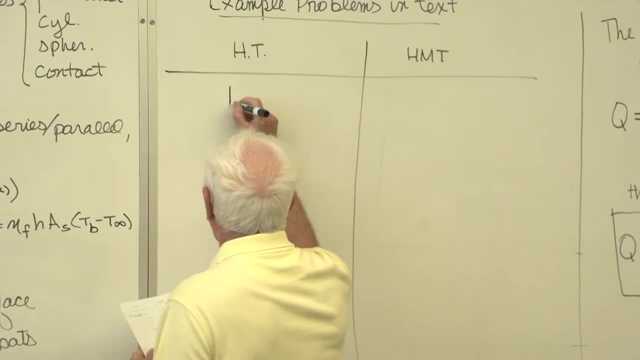 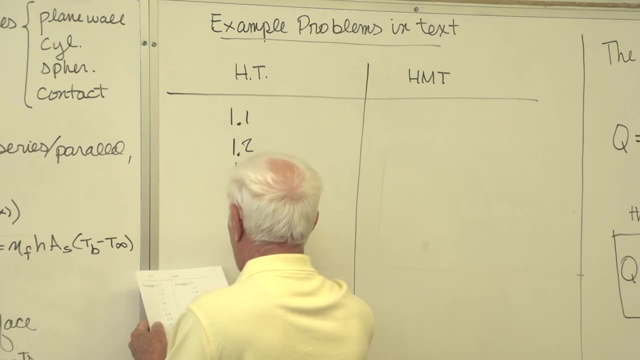 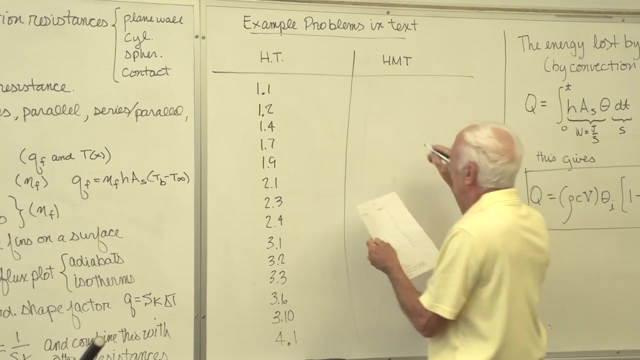 before the first midterm: Chapter 1, Chapter 2, Chapter 3, Chapter 4.. Now these same problems are in the heat and mass transfer textbook, but sometimes the numbers change because the author changed the textbook slightly. So these are the ones that are. 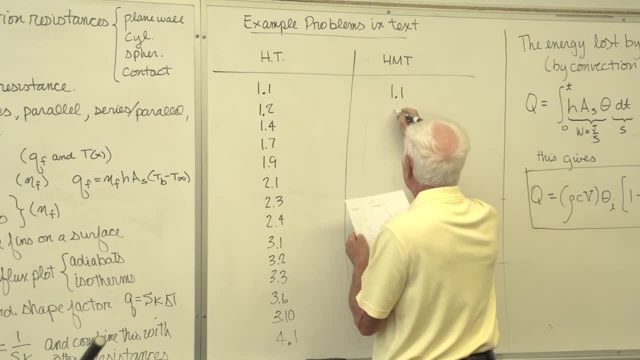 similar to the left-hand column, but they're in the heat and mass transfer textbook. It depends which one you've got in your hands or on your laptop. Most of the same numbers, but there's a couple of them that are slightly different. 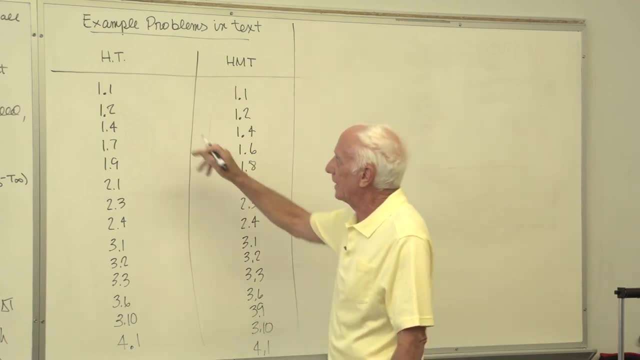 Okay, So you've got 1,, 2,, 3,, 4,, 5,, 6,, 7,, 8,, 9,, 10,, 11,, 12,, 13,, 14,, 2,, 4,, 7,, 9,, 1,, 3,, 4, right. 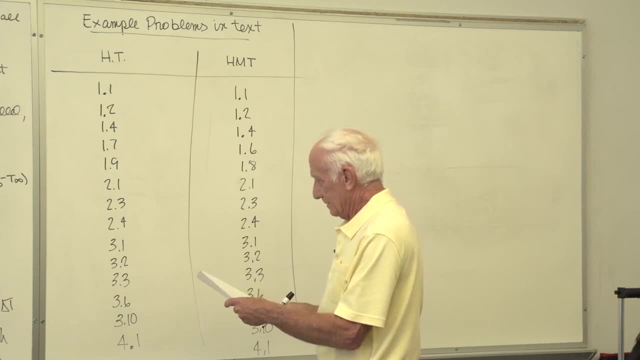 1,, 2,, 3,, 6, there should be okay, I thought I missed one- 6, 9,, 10, 3, 9,, 3,, 10,, 4, 1.. 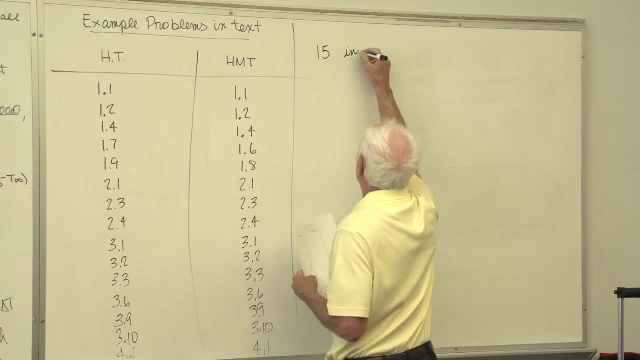 15 in-chapter work Examples You've worked: 18,, 24,, 5,, 6, 7,, 8, 9,, 10,, 1, 3.. Okay, Okay, Okay, Okay, Let's move up to chapter 7.. 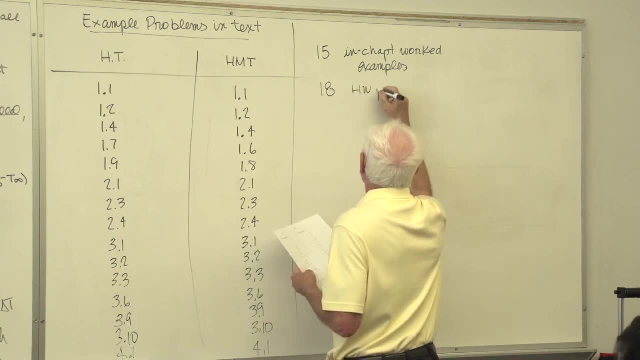 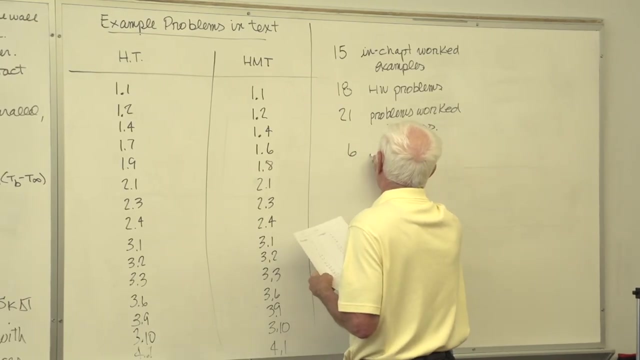 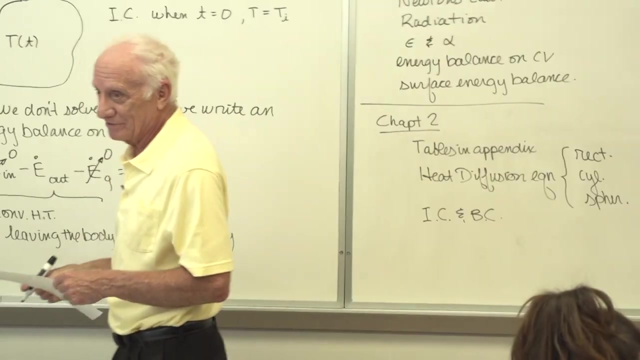 Let's move up to chapter 7.. homework problems. I've worked 21 problems worked in class. You got six previous exam problems, So you've got a library now of 60 problems you can review for the first midterm- 60 problems for the first midterm. 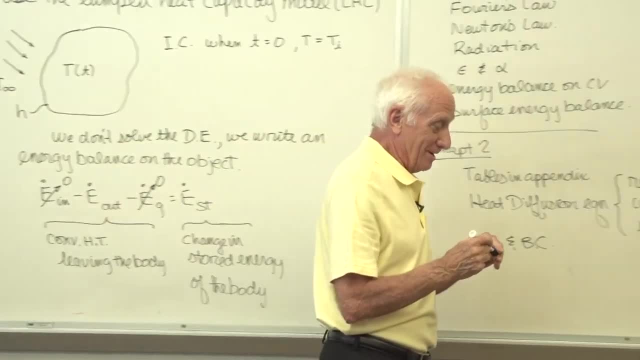 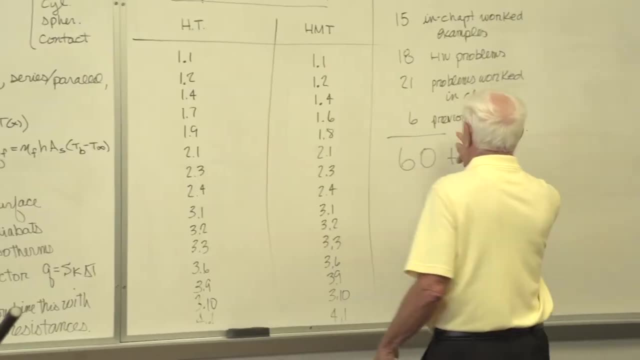 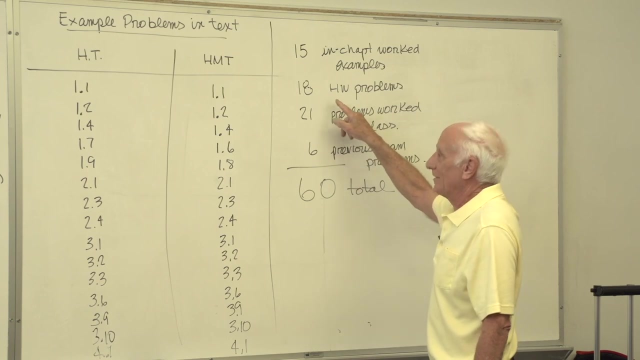 So, if you want to look at stuff, that's what you look at right there. What's most important? Well, obviously, what I asked for the last two years, that's that one. When I assign homework, why do I assign certain problems? 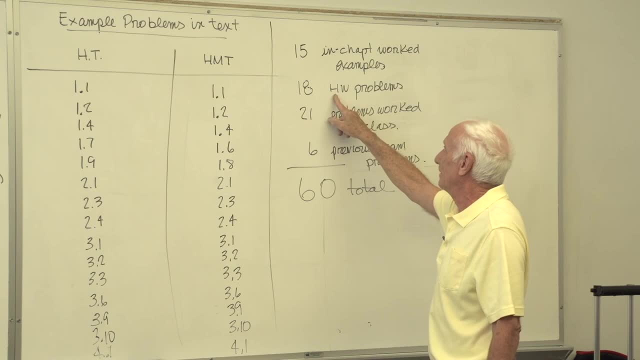 Because I think they tell a really good story. That's the next important one. What I work in class, because I want to go over that with you to see if you can understand what I'm doing up here in the board in class. This one here, this is the ones. 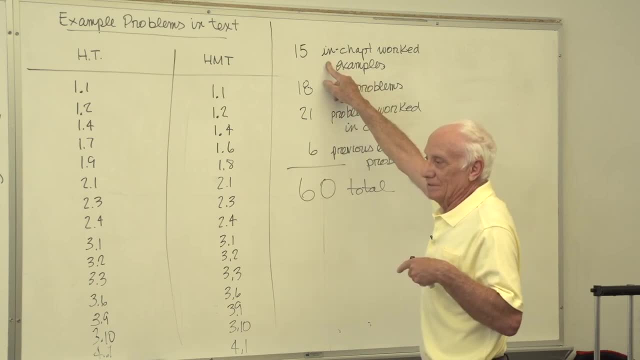 this is working class. This in Chapter 1, that's what the textbook author thinks are important. Okay, that's all right, but that's not number one on the list. This is number one. this is number two. this is number three. 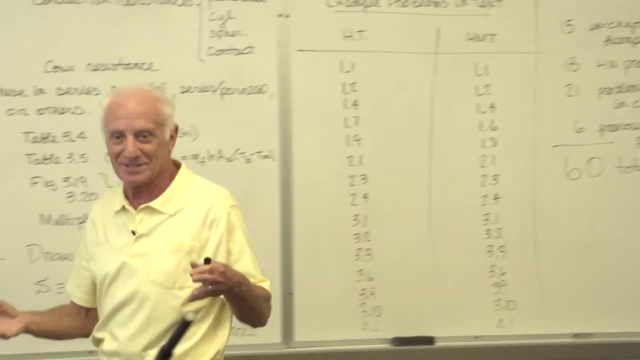 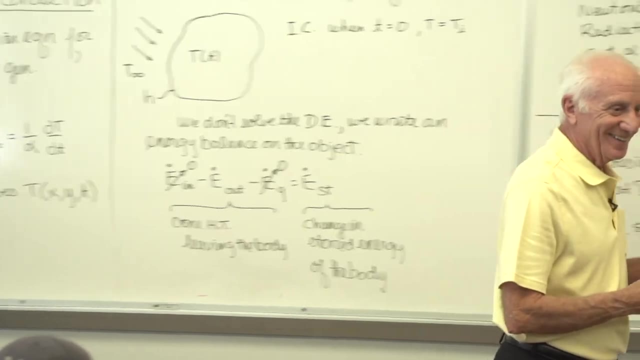 and that's number four. If you've got, prioritize your time for looking at stuff. That's what I would suggest. Any questions on that, then You know what you can bring to the test on Friday, what I'm going to give you on Friday. 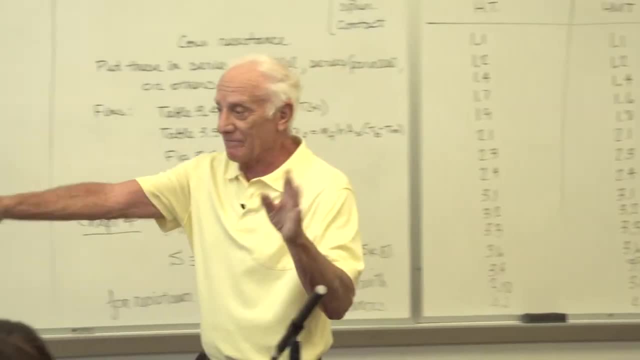 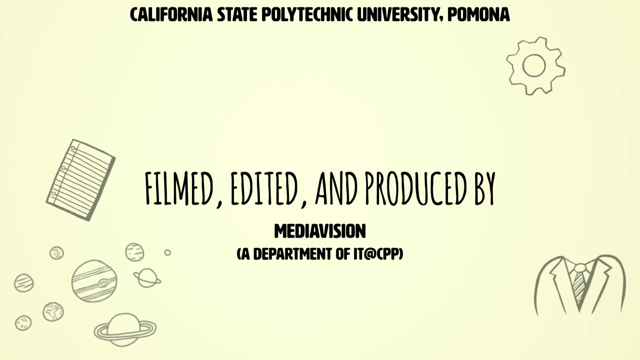 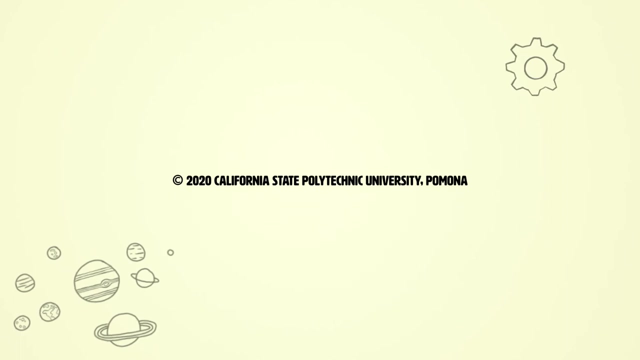 So we'll see you on Friday. then, If you have any questions, hang on around after class. I'll talk to you about any questions you have.